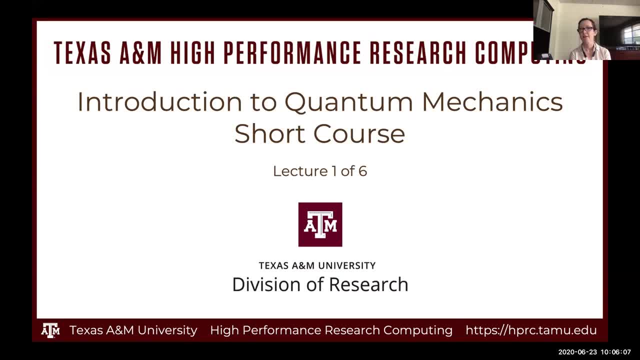 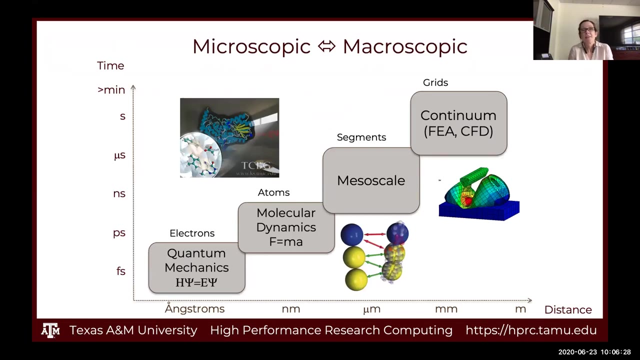 questions. you can post those questions in the chat and I will try to address them as quickly as possible. Okay, excellent, Thank you everyone. Okay, so before I get started in quantum mechanics, I'd like to give an overview of 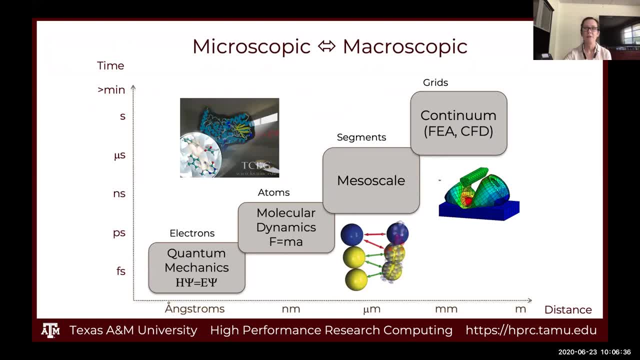 microscopic and macroscopic, just to show where we are going to be focusing. I'm going to get this here in just a second. I can get my pointer set. There we go. So I would just like to show where we're going to be focusing for this short course. 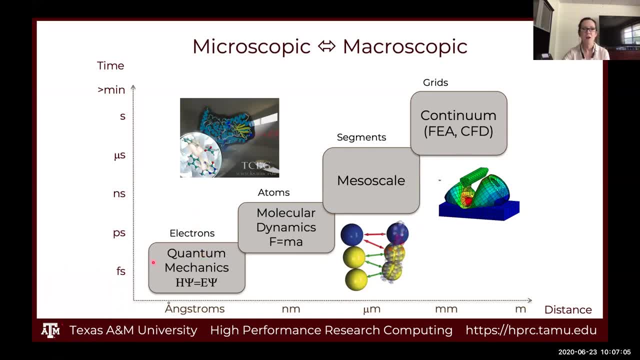 Okay, we're going to be all the way down here. We're going to be focusing on quantum mechanics, where we have inclusion of electrons. So this is very, very microscopic scale and we're going to be dealing with the angstrom level. okay, and essentially not really including time directly. 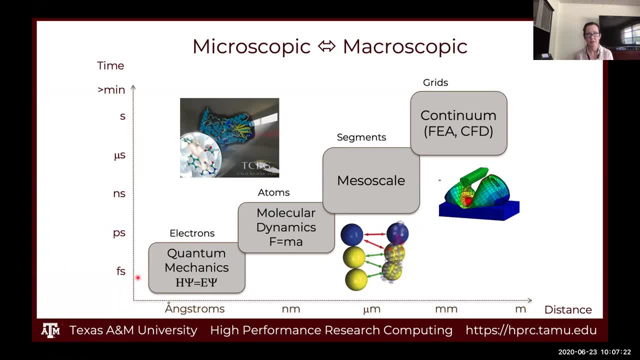 in these. So we're going to be dealing with the angstrom level and if you go up then you can maybe we'll talk a little bit about classical simulations, where you can maybe move up to the nanometer scale, you know, looking at large proteins. 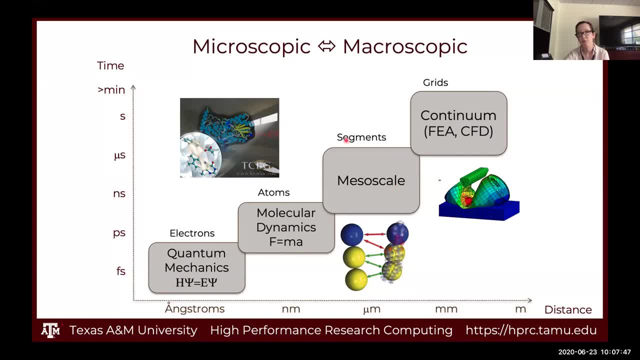 And then, if you scale up further, you can do something with segments where you're talking about the mesoscale, where you're no longer looking at the nanometer scale. you're looking at the nanometer scale and you're looking at the nanometer scale. 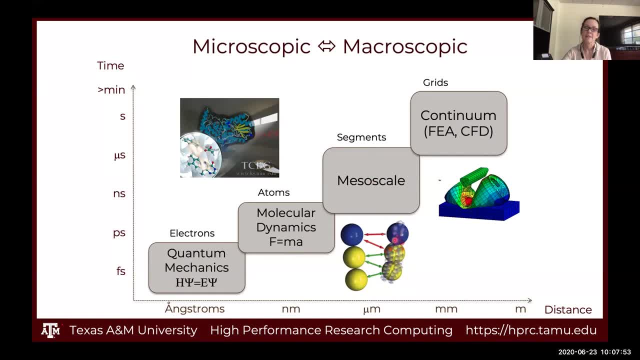 So we'll be dealing with that. So if you're looking at the atoms directly, you're looking at some segments, okay, and then going up further would be grids, where you're at the continuum level, where you can look at more of the macroscopic processes- okay, and going from here all the way up to here is still an area of development. 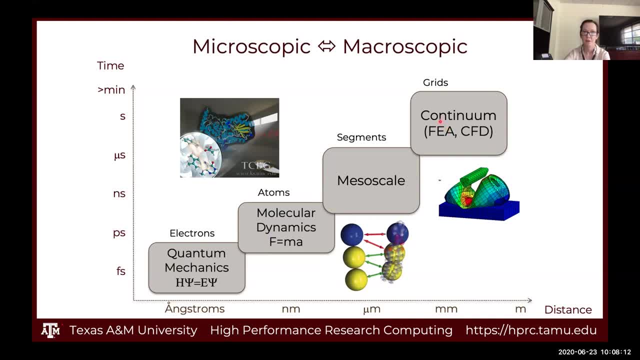 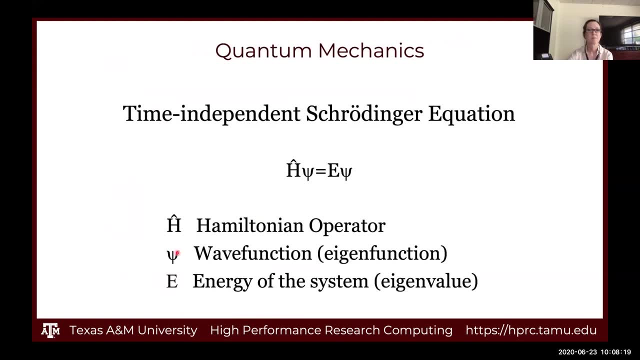 There's a little bit of overlap, but it's very hard to go from here to here, but today we will be focusing all the way down at the angstrom level. So what are we talking about when we're talking about quantum mechanics? And I'm sorry, let me backtrack just a little bit- 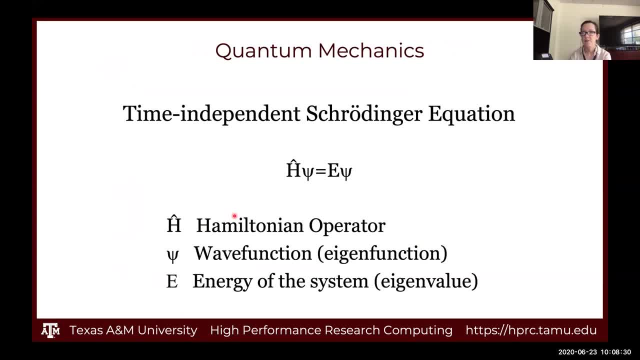 The goal of these lectures and hands-on sessions is to give you an introduction of the topic, some of the mathematics behind it and the caveats in those mathematics, the approximations that are made, some of the more important concepts that you will run into problems with when you try to apply it to your research. 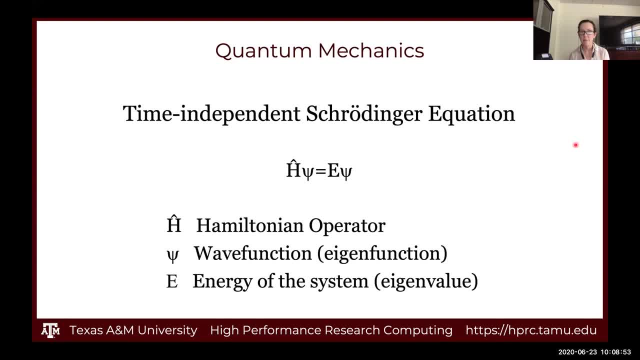 Okay, so that is the goal of this course. I don't expect anybody to be able to go out and just run their research with quantum mechanics without additional support. Okay, so it really is an introduction. Okay, so what we're going to be doing with quantum mechanics is we're going to try to solve this thing called the time-independent Schrodinger equation. 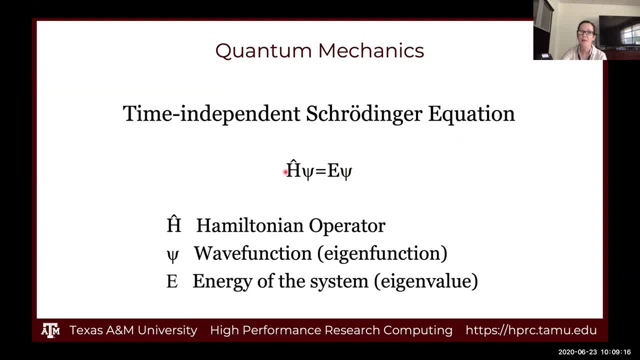 Okay, and this is an eigenvalue problem, We have this Hamiltonian operator. It's going to be operating on this thing called a wave function. Okay, It's the eigenfunction. It's going to give us the energy of our system. 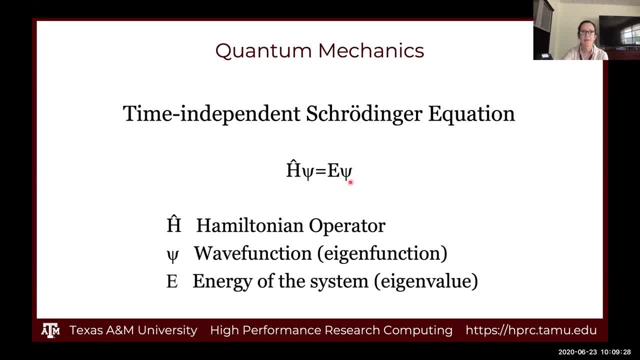 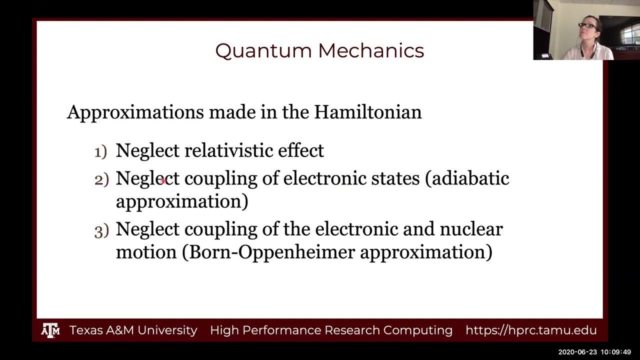 Okay. And then the wave function back again. Okay. so the goal of this course is to go over the forms of the Hamiltonian and the forms of the wave function that are used in traditional quantum mechanics calculations on molecular systems. Okay, so the first thing that we should talk about are the major approximations that are made in the Hamiltonian. 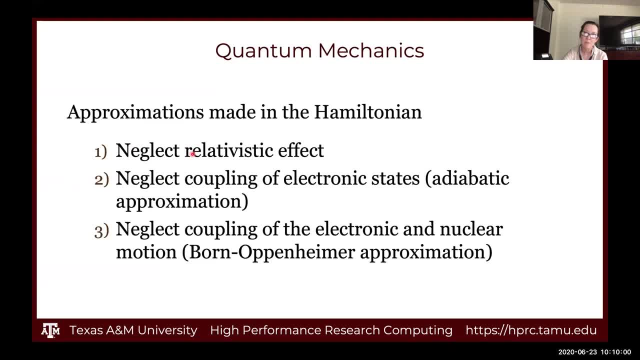 Number one is in the Hamiltonian. for the vast majority of calculations it neglects relativistic effects. We are going to incorporate relativistic effects in a different way, using something called effective coordinates. Number two is in the Hamiltonian for potentials, which we'll talk about in lecture two. 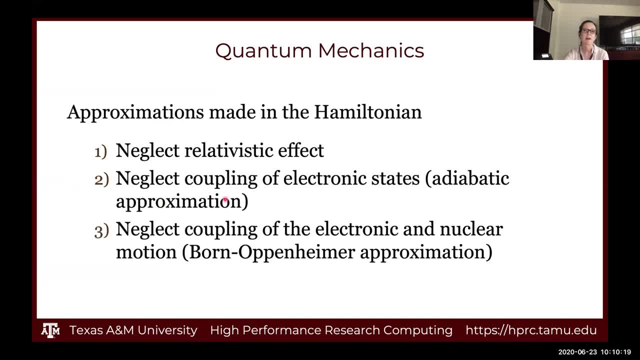 We're also going to be neglecting coupling of electronic states- This is called the adiabatic approximation- and we will be neglecting the coupling of electronic and nuclear motion. This is the widely known Born-Oppenheimer approximation. Okay, so what does the Born-Oppenheimer approximation mean? 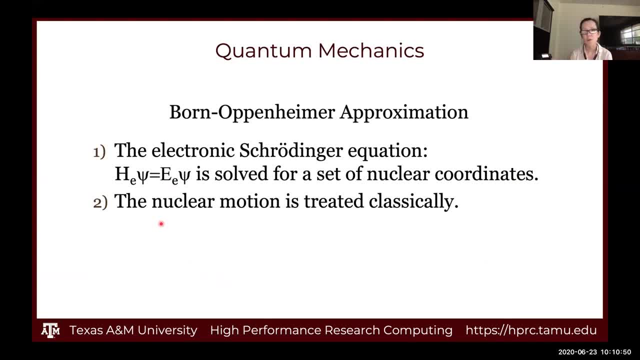 Right. so we're going to be solving the electronic Schrodinger equation, We're going to completely decouple the nuclear and electron motion and we're going to solve them parametrically. So since the electrons move substantially faster than the nuclei, we make the grand assumption that we can treat them somewhat independently as far as their motion. 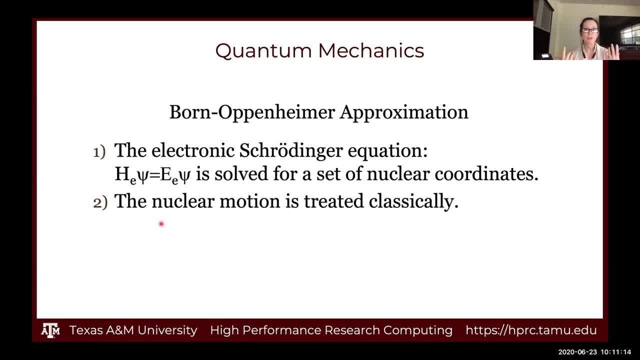 Okay. Okay, We can split up the equation and we can just solve the electronic Schrodinger equation. So the electrons are seeing static nuclei, nuclei that aren't moving. In reality they're coupled. but this approximation is generally okay. 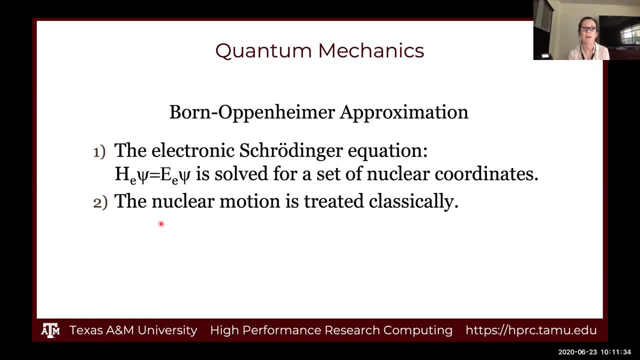 It's not always okay, but for the vast majority of calculations it's okay. It is one of the major approximations that's made in the Hamiltonian for most molecular quantum calculations Okay. So we've completely decoupled them and we solve them parametrically. 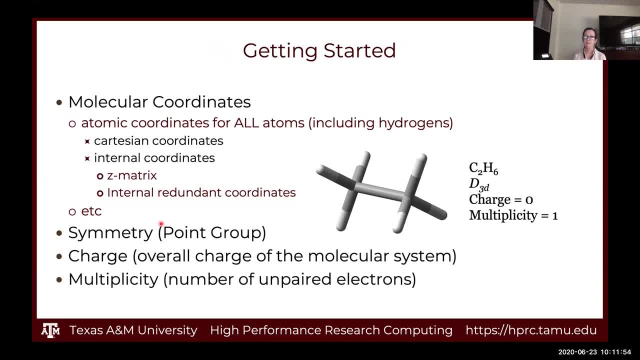 Okay. so the first thing that we need to do to get started in performing quantum calculations is you need to have molecular coordinates. Okay, all of the molecular coordinates, including the hydrogens, And I've seen this over and over and over again. 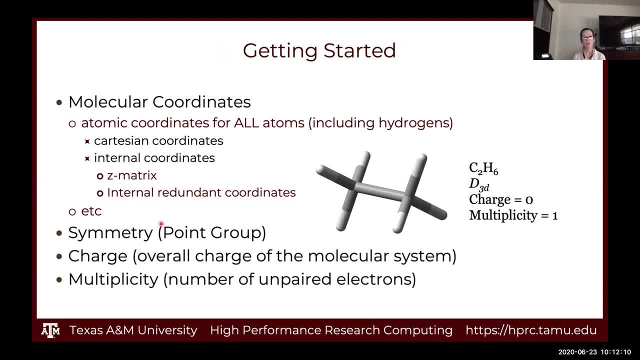 People will start with their calculations and they'll go get a structure or they'll draw something And they won't have all the hydrogens in place, Or they will have a catalytic reaction. They throw some stuff in there and want to do calculations on it. 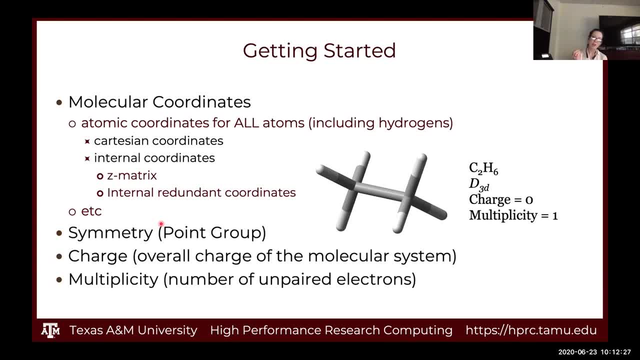 You have to have intimate knowledge of the atomic coordinates for your molecules if you want to do molecular quantum calculations, Okay. So you have to have a good starting structure, reasonable coordinates for all of them, All of the atoms, including the hydrogens. 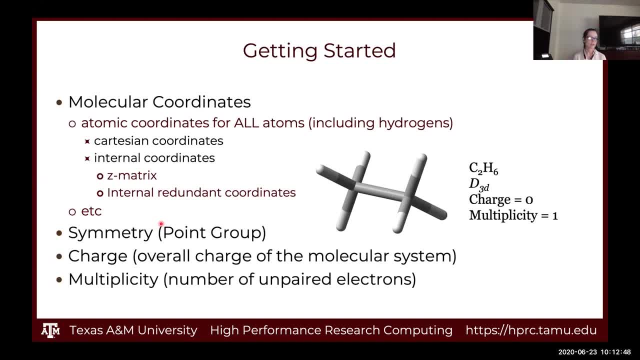 Okay, you can provide these coordinates in many different ways: Cartesian coordinates, internal coordinates, Z matrix, internal redundant coordinates. There's a long laundry list that you can usually provide, but you have to know the element and where it is in space. 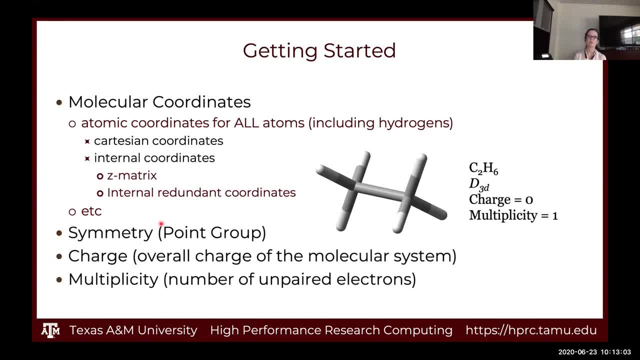 Okay, relative to each other and all of the elements involved. So this is an example of ethane. right, We have C2H6.. We're going to talk a little bit about C2H6.. We're going to talk a little bit about symmetry. 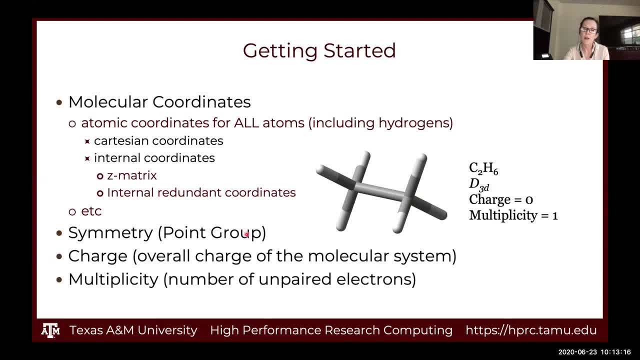 This has D3D symmetry. You should know if your molecule has symmetry. This has an impact on the calculation, which we'll talk about more. You're also going to need to know the overall charge of your molecular system. Okay, so for this one, the overall charge is zero. 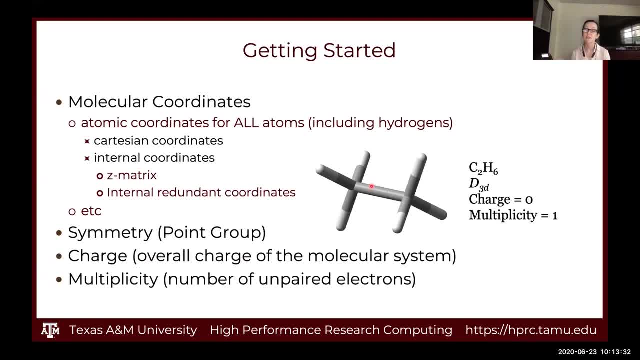 So a lot of people will automatically want to assign charges to each individual atom. Okay, in the quantum world, the electrons, they're shared. Each element may hold a charge, Okay, Okay, Okay, A larger percentage of that electron, but the electrons are shared. 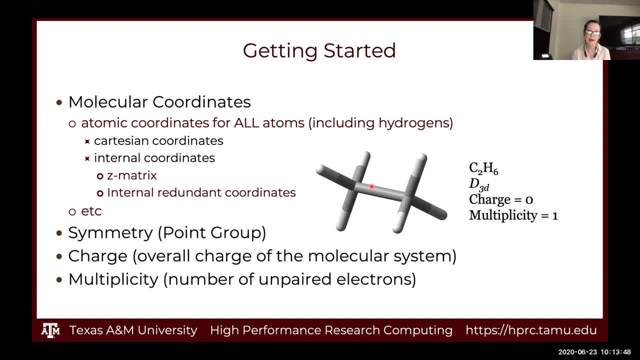 So we don't assign charges to the atoms, We give an overall charge, which is the electron count for the system. The other thing that you need to know is the multiplicity, the number of unpaired electrons. So in this case our multiplicity is one because we have no unpaired electrons. 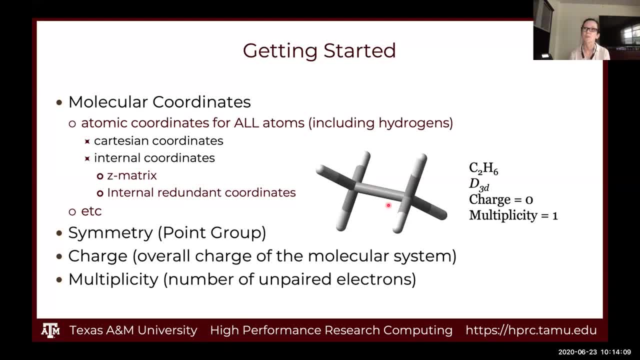 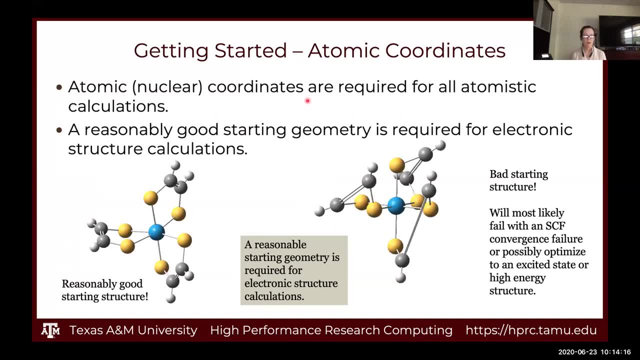 And we'll get to the definition of multiplicity at the end of this first lecture. Okay, so getting started with the atomic coordinates, like I said you need to have. you have to know all of the elements, where the hydrogens are, where everything is in space, but you also need a good starting structure. 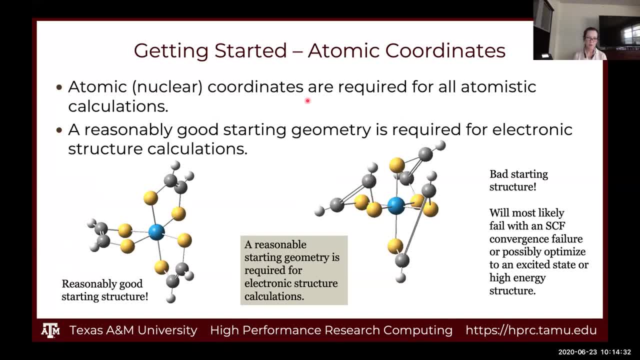 So if you don't have a good starting structure, you will end up either having something called an SCF convergence failure Or you will, Or you will optimize to an excited state or some other high energy structure that's not pertinent to the chemical system that you're interested in. 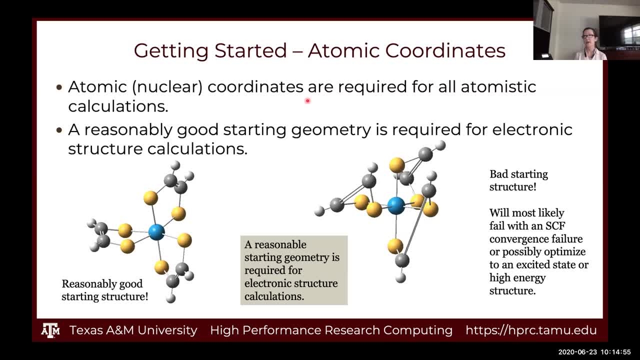 Okay. so where you get your reasonable starting structure really depends. If you have a crystal structure, that's a good place to start. However, lots of crystal structures have disorder, Okay, which means that they have atoms that are either in multiple locations because they have 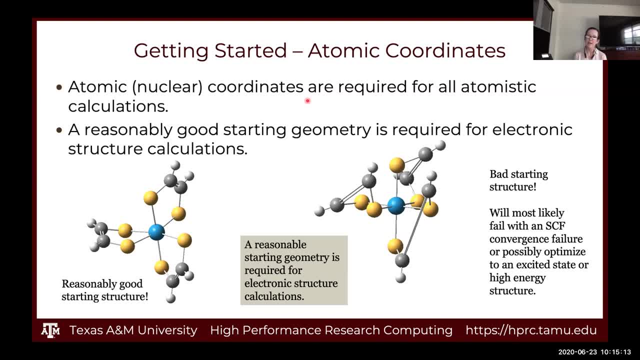 Two occupancies and you have to clean that structure up. and the other issue with the crystal structures or the hydrogens. Addition of hydrogens to crystal structure sometimes is not correct- Okay or poorly done, or they're left off completely Okay. so you have to clean up all of that to provide to the calculation. 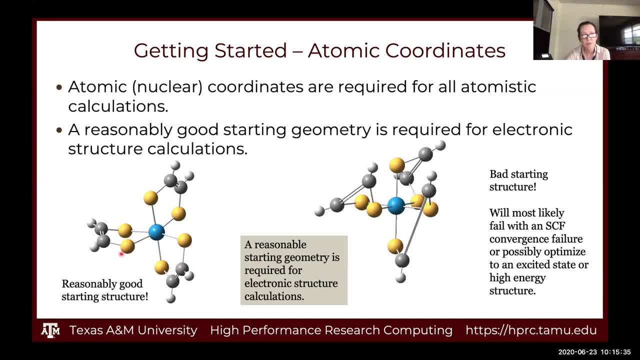 Okay, so here's just an illustration of a reasonably good starting structure, And this is a bad starting structure. Now you'll notice there are bonds. There are bonds drawn Right. when it comes to quantum calculations, you can draw bonds all day long. 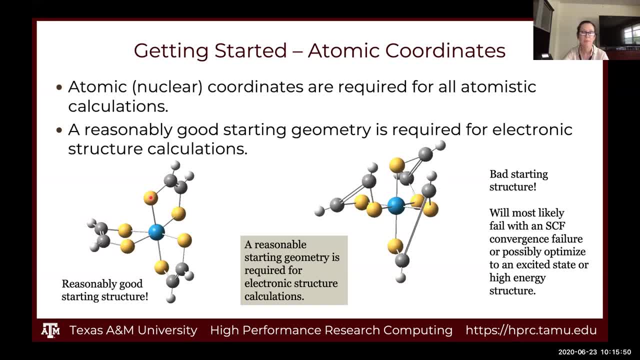 It means nothing. It means absolutely nothing because it's going to optimize the wave function, which is going to localize the electrons. It cares nothing about what you draw for bonds. It only cares about where this atom is relative to this one, what the distance is, what the angle is. 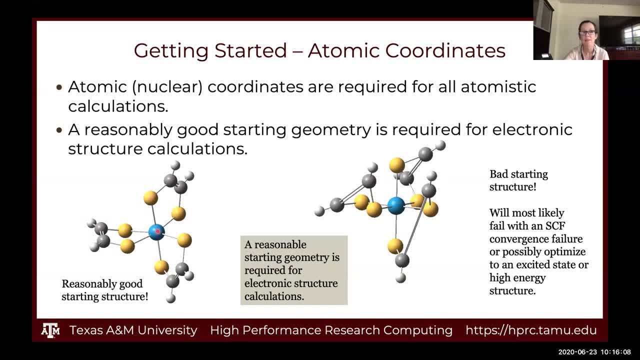 Okay, because it's the proximity of this atom to this atom that lets it Develop the atomic molecular orbitals and optimize the wave function. Okay, so, even though I have, you know, a double bond drawn here and a double bond drawn here, this is a bad structure because this distance is unreasonable. 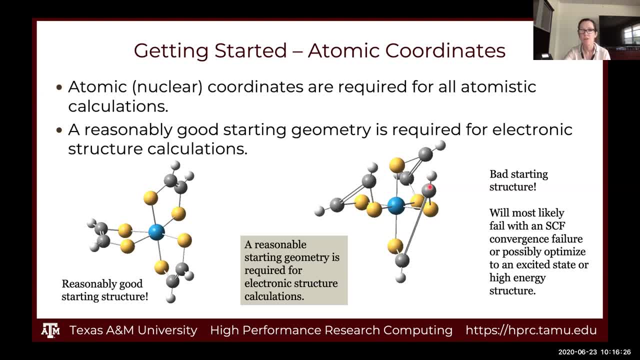 And it's not going to be able to optimize a wave function, or if it does, it's going to be a very bad wave function. Okay, so you really need a good starting structure. If you don't have a crystal structure, there may be a similar crystal structure that you can start with. 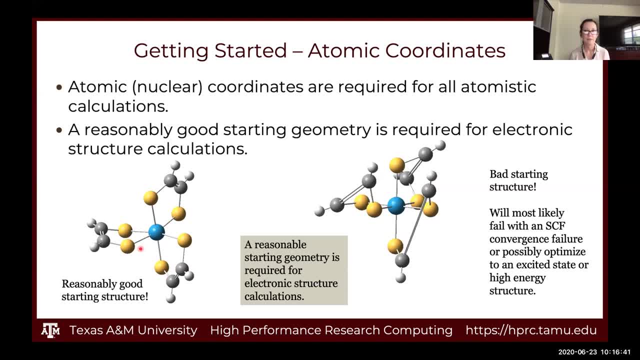 Okay, so you really need a good starting structure. If you don't have a crystal structure, there may be a similar crystal structure that you can start with And then modify it with your favorite drawing program. There's a ton of them out there. 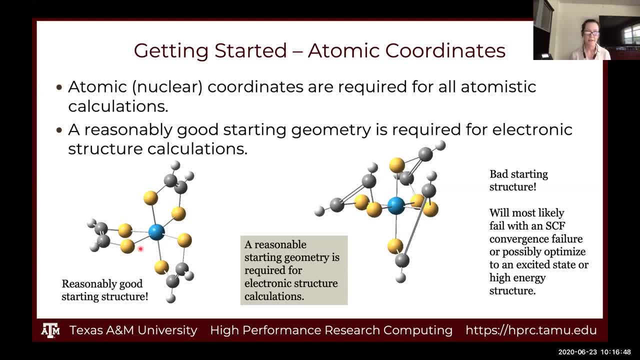 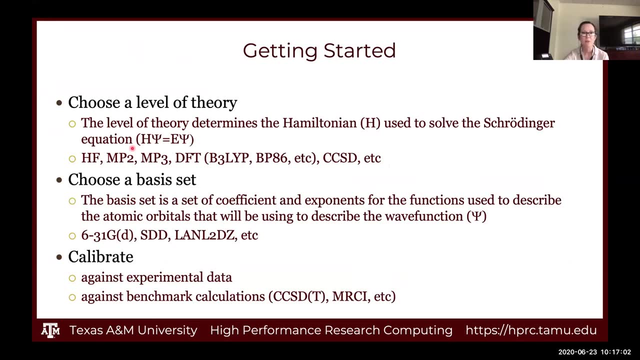 Okay, so you can find your favorite drawing program and draw it in there, Okay, and it takes a little bit of getting used to and it really depends on the type of system that you're going to be investigating. Okay, so this is my general overview. after you have your molecular system, 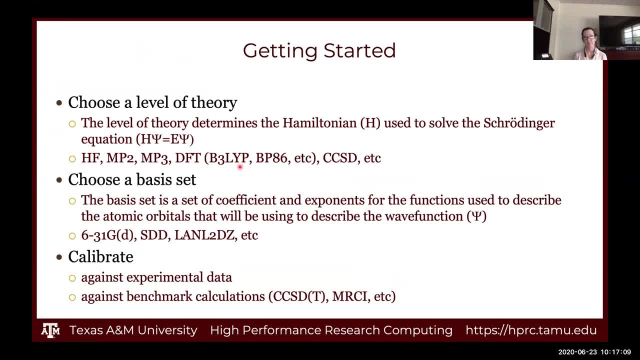 Then you have to decide about a level of theory. Okay, the level of theory will determine the Hamiltonian that's going to be used for the Schrodinger equation. So remember, we're doing our time-independent Schrodinger equation and we have this Hamiltonian. 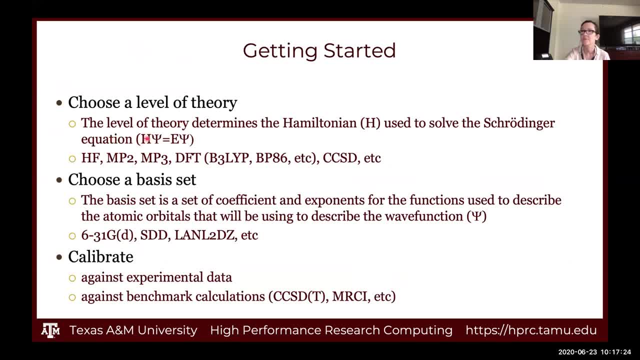 Okay, the level of theory determines the form of the Hamiltonian. There's a lot of them that are out there: Hartree-Fock, Mulder-Placid series, density, functional theory, coupled cluster and more. So which one you choose, it really depends. 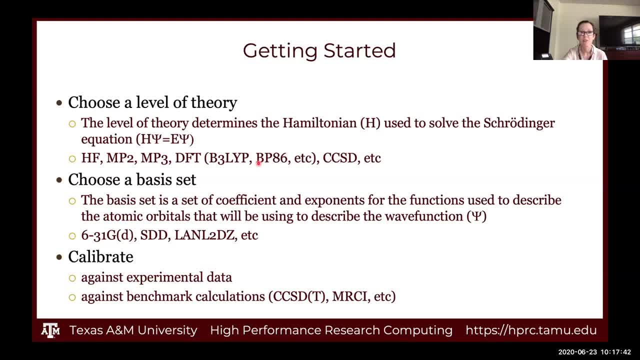 Usually, literature is the best place to start to see if somebody has already investigated your system type and determine what level of theory is best for it. Sometimes your choice of level theory also goes to computational cost. What can you afford to calculate? Okay, and we'll talk more about that later also. 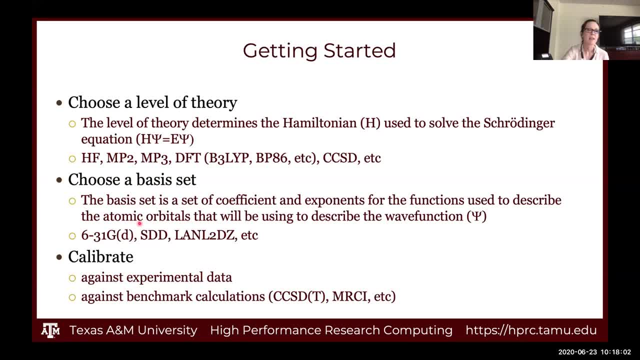 Then you also have to choose something called a basis set. So the basis set is going to determine the mathematical form of the wave function. So the basis set is going to determine the mathematical form of the wave function, and the basis set is going to determine the mathematical form of the wave function. 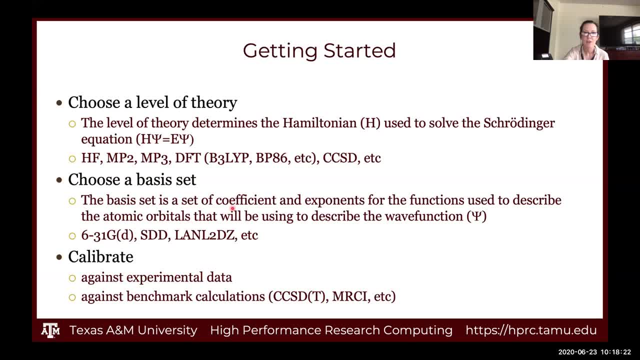 There's a lot of different basis sets out there. This is going to be a linear combination of atomic orbitals and we're going to discuss this more during the second lecture. It's the coefficients and exponents for the functions that are used to define the atomic orbitals, which get combined together to make molecular orbitals. 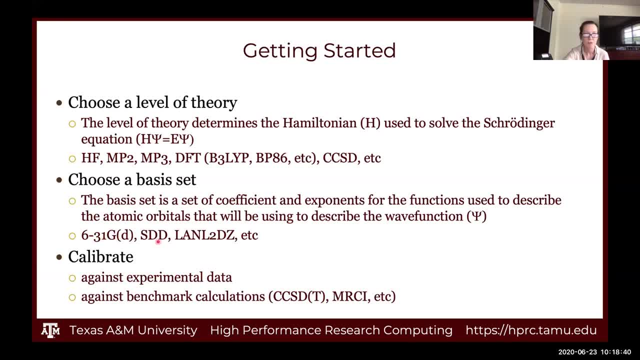 Okay, you'll see a lot of acronyms: The Popol style basis set, Stuttgart. there's a long list of basis sets. Again, how do you choose one? Literature is always a good place to start And, more importantly, calibration. 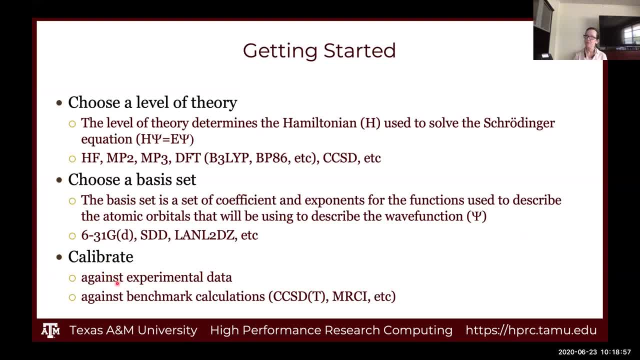 So you can do calculations, you can do calculations and you can do lots of calculations. but because there are substantial approximations that are made in these levels of theory, you need to calibrate Okay One. often you don't even know if the molecule that you're calculating is truly the molecule of interest. 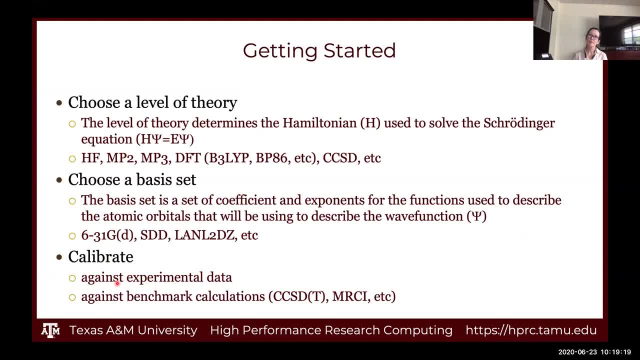 Okay, so you need to have generally some experimental data to calibrate against whether that be a crystal structure. if you have some rate information- UV-Vis- there's a lot of different experimental data that you can use to calibrate against. 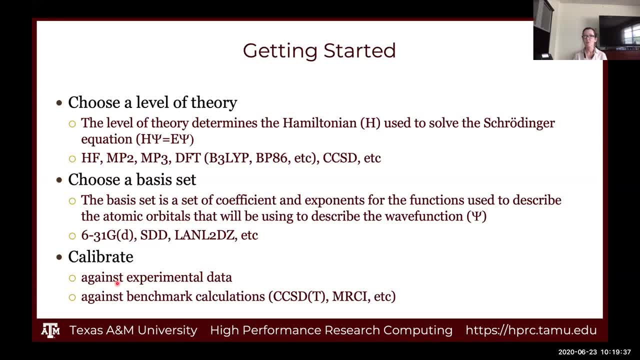 You can also calibrate against what are called benchmark calculations, Which are very high level calculations. So often what you do is you run a lower level calculations on a bigger system And then you might prune it down, run it again on that low level and then run it on the high level calculation and see if you're getting consistent results. And that's how people are often calibrating against benchmark high level calculations. 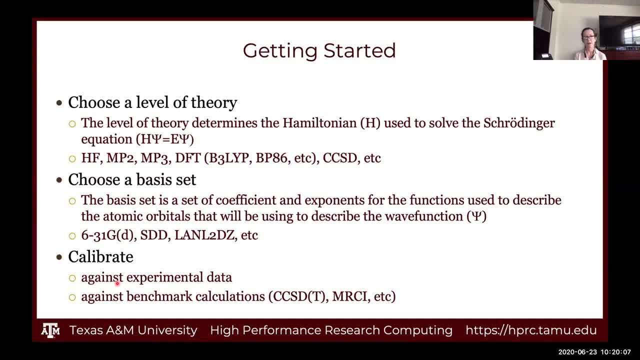 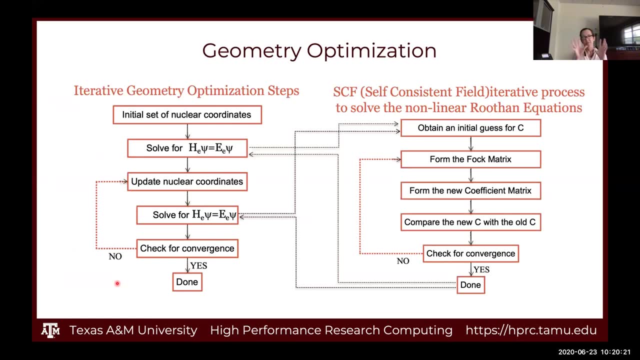 I believe that we're going to get to the benchmark level calculations. I'm on day two or might be day three. I can double check that. Okay, so the general. when you're getting started, I said you need a good starting structure. 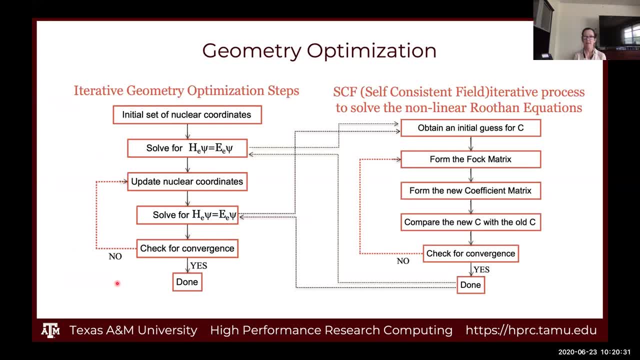 If you don't have a good starting structure, you're probably going to end up getting something called SCF, convergence failure. So the vast majority of these calculations will optimize the wave function that we're going to be solving for By doing a self consistent procedure, And that's what's illustrated here in this flowchart. Okay, this iterative process, It's called SCF. Okay, it's solving a set of nonlinear equations, Right? So the first thing that it has to do is obtain an initial guess for this thing called C. 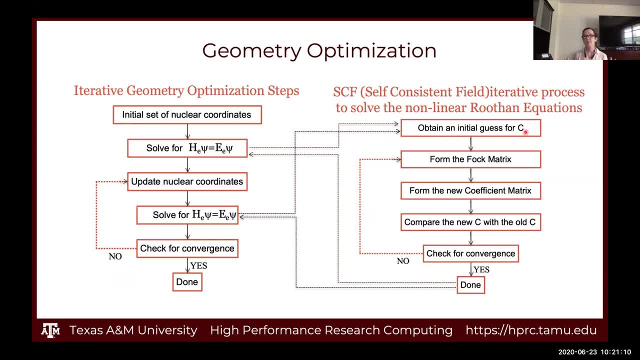 The C is your coefficient matrix. This is the coefficient that is part of the basis set that goes to the atomic orbitals. So if you have a really bad starting structure it's going to have a really hard time assigning a reasonable initial guess for the coefficient matrix. 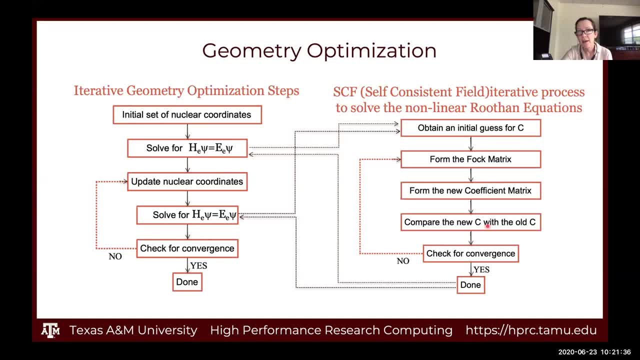 So if they can't assign a good coefficient matrix, then it's going to fail When it goes through this iterative process. it's not going to be able to optimize the wave function. Okay, so we're going to revisit what each of these steps means. 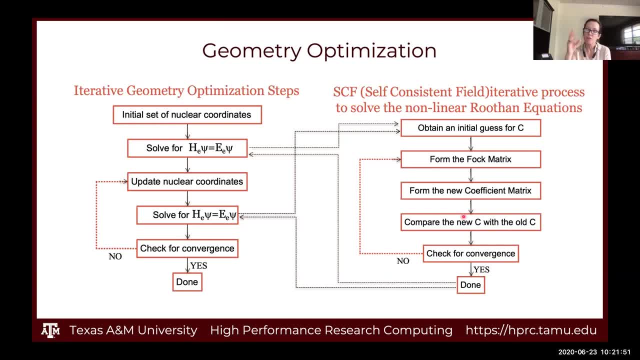 But I wanted to illustrate that it's an iterative process and you're starting. geometry is critical for getting a good initial guess, Which is critical for optimizing the wave function. Okay, so it goes through this process of optimizing the wave function. Once it gets the wave function optimized. 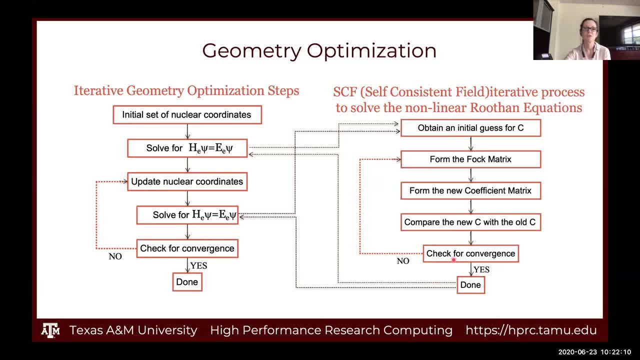 Then it will go through and do a geometry step and then the wave function and then the geometry. And this also goes to the Born-Oppenheimer approximation Where we have decoupled the electron and nuclear motion. So here we're optimizing the electronic part and here we update the nuclear coordinates and then the wave function and then the nuclear coordinates. 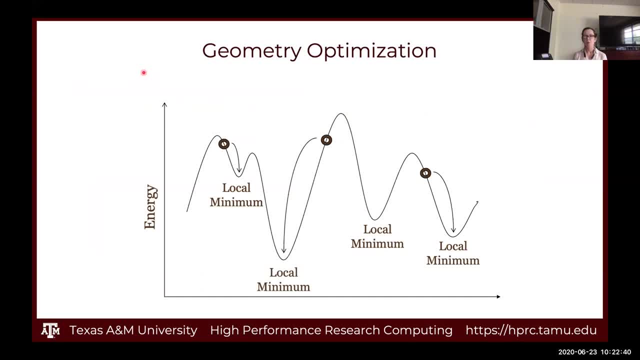 So, as we're updating the nuclear coordinates, I'd like to point out: if you're going to be optimizing the geometry of your molecule, Your starting structure is critical, not just for getting a good wave function and getting the wave function to converge, but also where you're going to end up on the potential energy surface. Okay, so this is just a schematic representation of something called a potential energy surface. 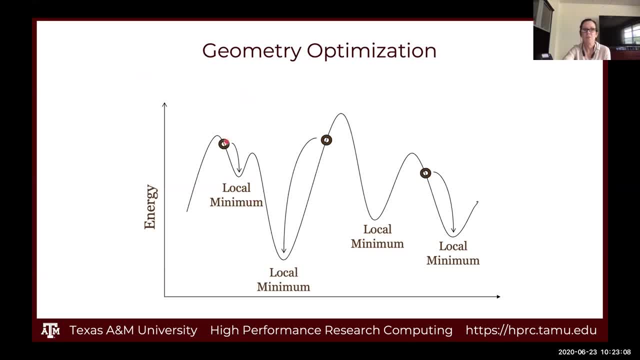 When you're performing a geometry optimization. If you start with a molecule that has a geometry that is somewhere like this on the potential energy surface, you're going to fall into this local minimum. If you start here, you'll fall into this one. If you start here, you'll fall into this one. 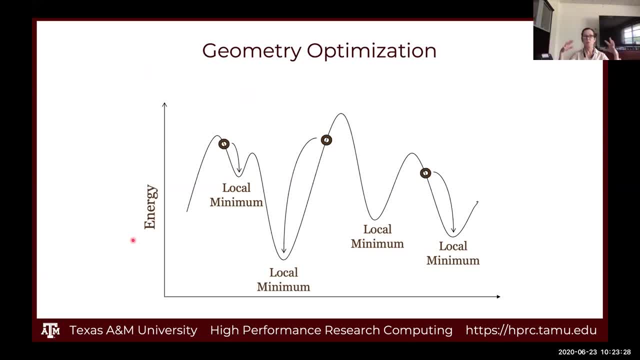 So you can. if you have a big floppy molecule, when you perform a geometry optimization, just a standard geometry optimization- it's not going to sample conformational space, It is not going to move the ligands around substantially and look for lower energy minima. It's only going to optimize to the closest minimum of your starting structure. 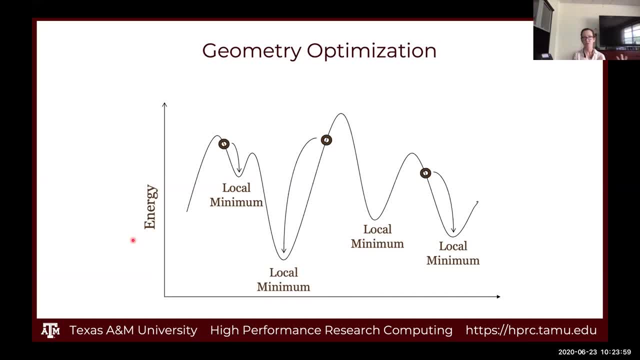 Okay, which may or may not be the confirmation or structure that's important for your experimental results. Okay, So you need to keep in mind that it's only going to optimize to the closest minimum and it's not going to sample different confirmations for you. There are other procedures if you want to sample conformational space, but a standard optimization does not do that. 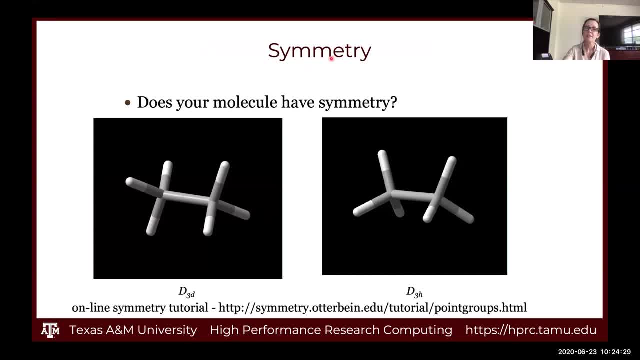 Okay, so does your molecule have symmetry? Symmetry is very useful for quantum calculations because it can decrease your computational cost. These calculations are computationally intensive, So that means they use a lot of memory, It uses a lot of CPU and they run for a long time. 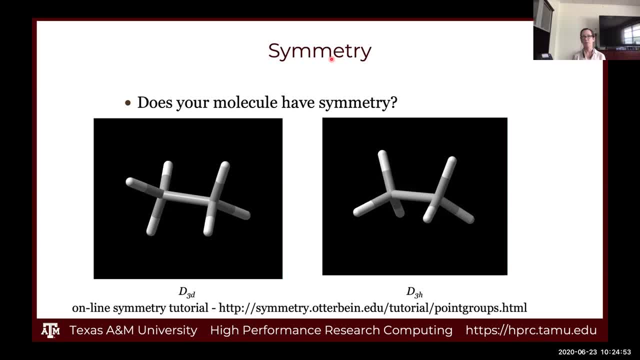 If your molecule has symmetry it can decrease the amount of computing that it has to do. For each symmetry element it halves the computational cost. So it is beneficial to use symmetry. but you need to be careful because if you have symmetry-imposed which is 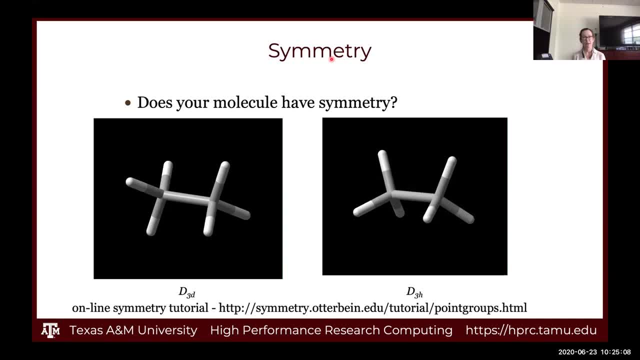 the correct symmetry, most likely it's going to maintain that symmetry and you're going to get the wrong result. Okay, so here's my simple Fane example. We have something called D3D symmetry for the staggered conformation, and we have 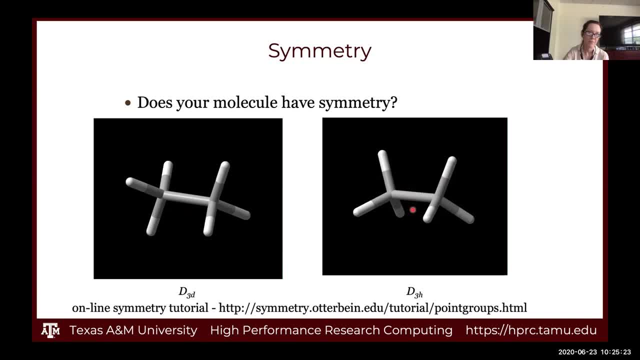 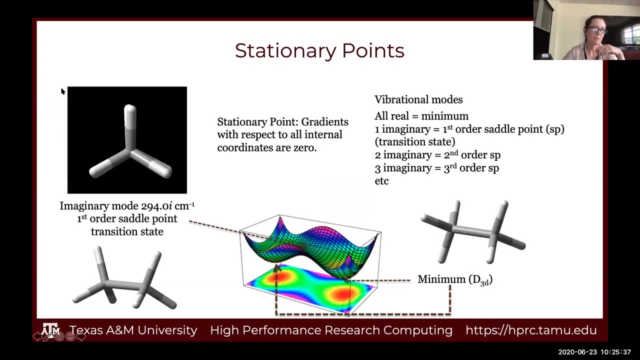 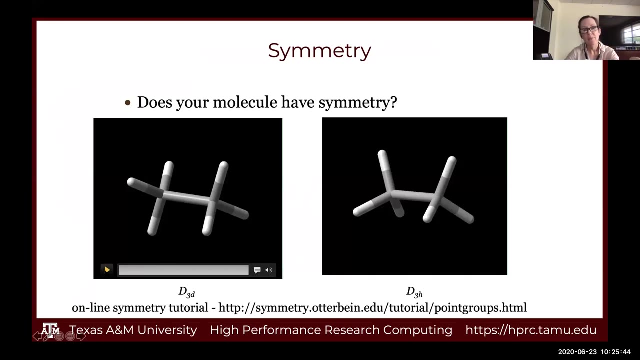 D3H for the eclipsed conformation. So if you're performing a geometry optimization for this and my movie is not working, so let me. I'm gonna exit for a second. Yeah, it won't work when I'm doing the laser. Okay, so when I'm playing. 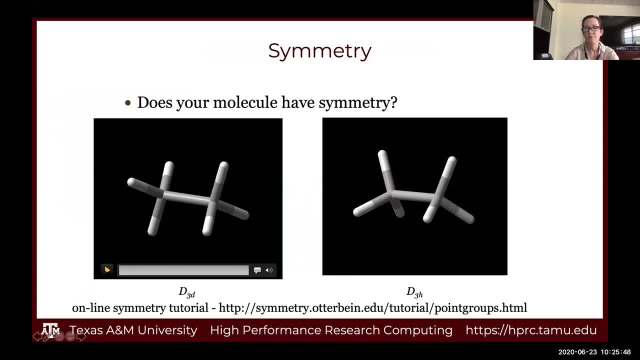 this. that's how much change there is in the optimization. This is a geometry optimization. it's my starting structure. that's my ending structure. Okay, so there's not a substantial change. I go to the D3H. Okay, again, there's not a substantial change. Okay, so let me ask. 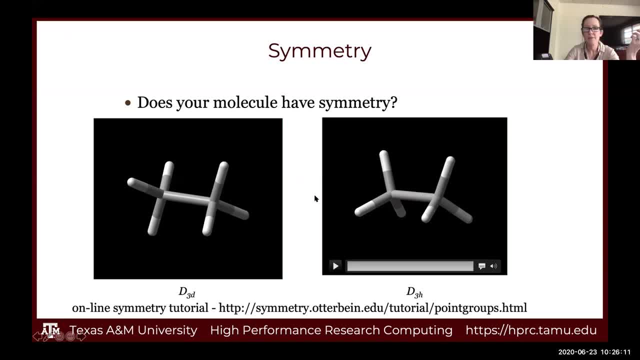 those in the audience are both of these minimums? are both the D3D and the D3H staple species intermediates? are they minimum? I'll 길 just a minute for everybody to think about that. Okay, so the staggered conformation for Fane is the stable species. 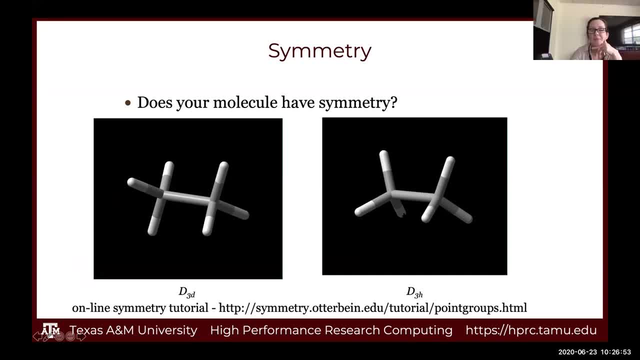 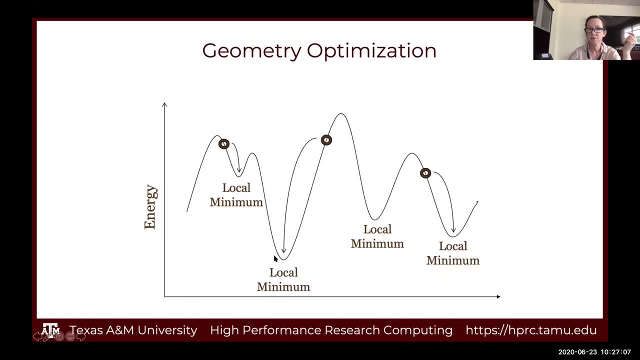 It's an intermediate or reactant, okay, This is a transition state. This is a high energy point on the potential energy surface. So if I'm doing a geometry optimization that's supposed to optimize to a minimum, if I come back to here, geometry optimization standard should go to a. 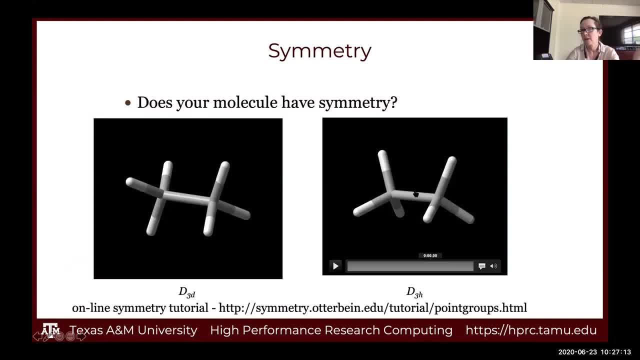 minimum. Why didn't I get a minimum with this one? It's because I imposed symmetry. So this is where the danger can come in, if you impose the wrong kind of symmetry. Now, this can also be helpful when you're trying to calculate a transition state, the high energy point on the 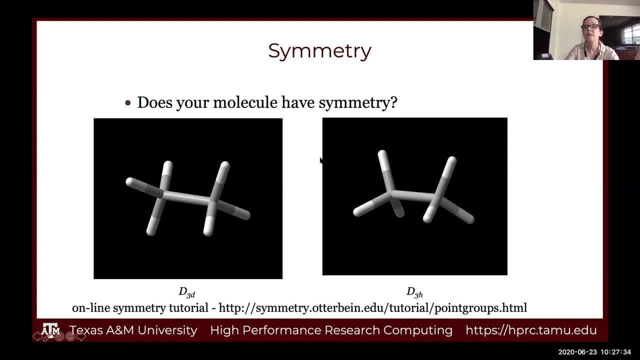 potential energy surface for a reaction. But you need to be aware of symmetry that's imposed for the system. So I think there's a question in the audience. how can you tell We're going to get to that? So the question was: how can you tell if something is an intermediate or if it's a transition? 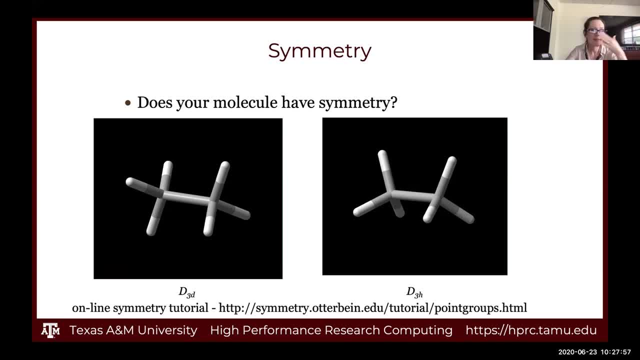 state. So if you don't have a chemistry background, there's something called a frequency calculation, which we're going to cover, I think, in a couple of slides that will tell you whether or not it's an intermediate or a transition state. So the point on this slide is that symmetry is very 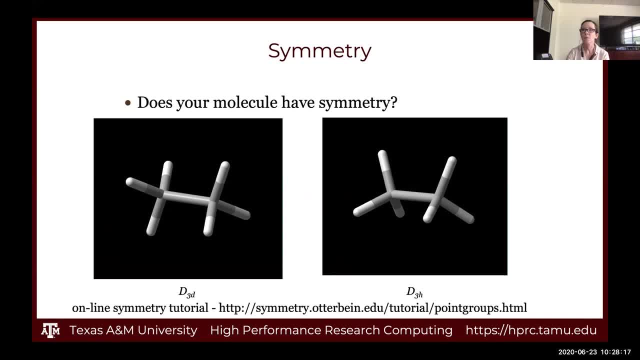 useful decreases your computational cost. but you need to be aware as to whether you impose symmetry and you need to double check to make sure whether or not you've optimized to a minimum or some higher order saddle point If you do not have a background in symmetry for molecular species. 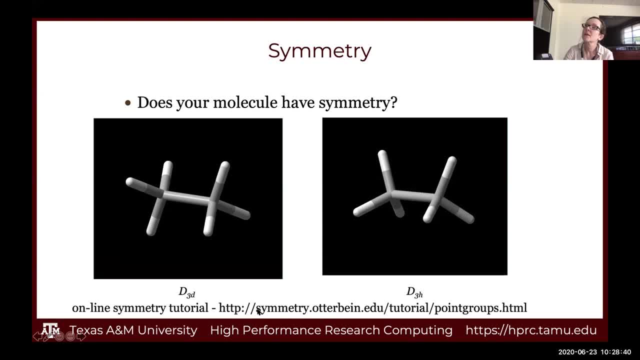 this is a very nice online tutorial. Okay, So there was a question that the hydrogens are much closer to the opposite hydrogen. Yes, they're in the eclipsed form. It's not where they want to be. Okay, This is staggered. They're further away. 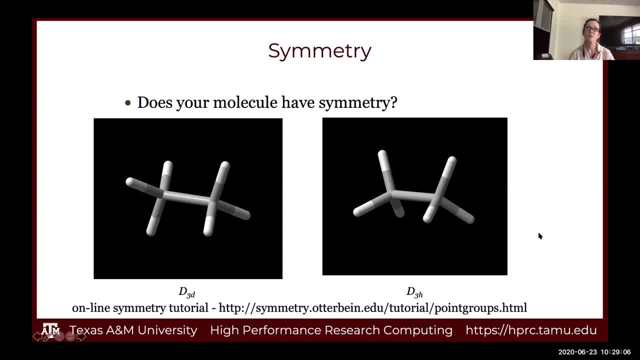 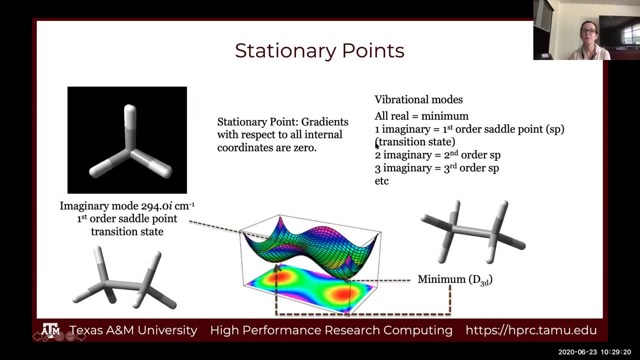 And we can also ask more questions and go over some of these things during the hands on session. So I'm going to be throwing a lot of information at you. That's why there are six lectures And this is just the getting going. Okay, so this is the slide that goes over more about the stationary points. Okay, 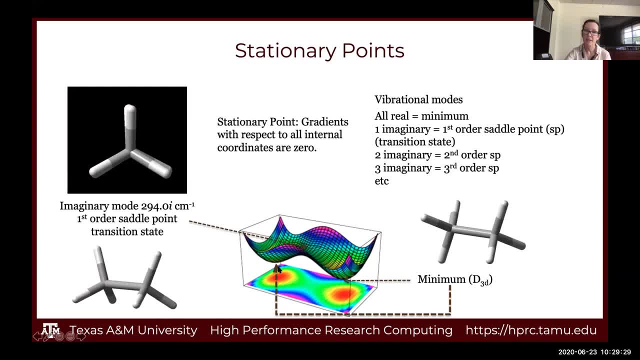 So I talked about the minima on that fictitious potential energy surface. Okay, so this is another representation of a potential energy surface, Okay, in three dimensions, where we have a minimum here and we have a minimum here, and for the reaction to go from one minimum to another, you go over this point right here, which is the transition state, Okay. 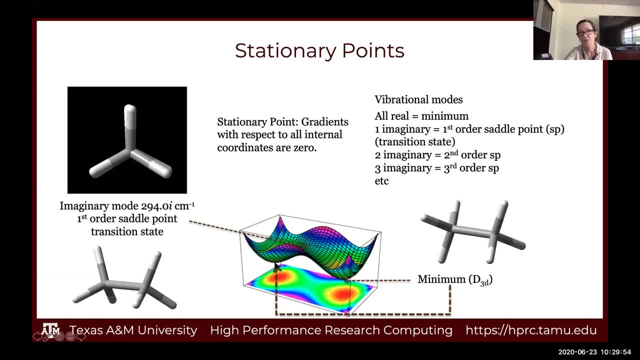 So to determine what kind of point you've optimized to, you can do a frequency calculation. The frequency calculation will give you the vibrational modes And if you look at the vibrational modes, if they're all real, you're at a minimum. 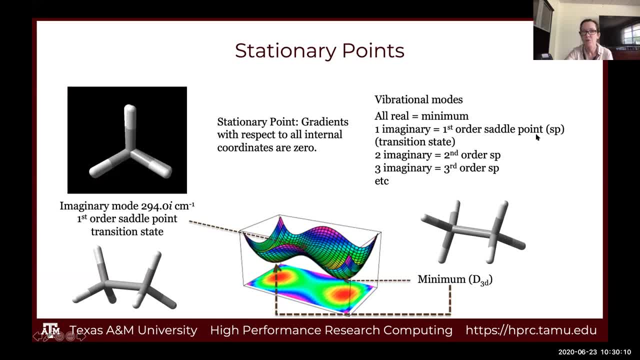 If you have one imaginary mode, then you're at something called a first order saddle point, which is the transition state and transition state theory. If you have more than one imaginary mode, you're at some higher order saddle point that is generally not on the reaction path. There are some specialized things where you have vibrational modes. 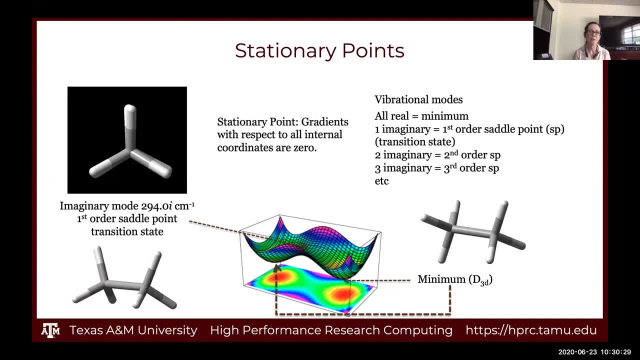 Okay, that's from my reference data. Okay, All right. so what am I doing here With a transition state theory? that's basically a Defrag foreseeable moment, Okay, So let's deep dive, deeper, All right. So, for example: Okay, 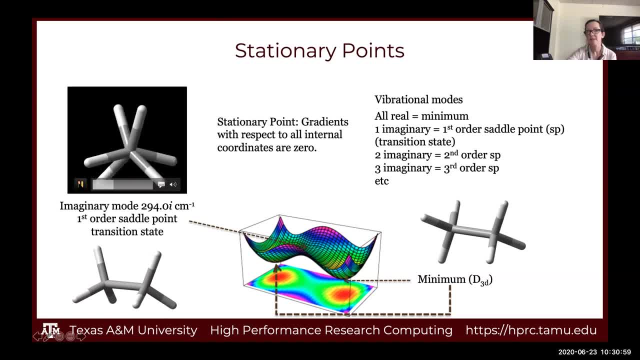 This is the recursive cannonsballs. Okay, d3h. This is the imaginary mode, It's the imaginary frequency and it has that twisting motion that connects the two minima. So whenever you calculate these, you always want to look at the imaginary mode to make sure that it is consistent. 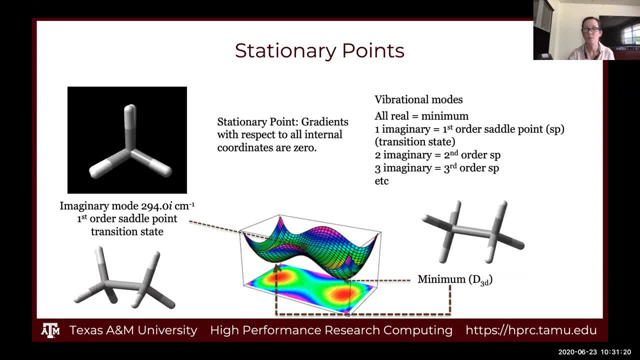 with the transition state that you're expecting to find. If it is not consistent, I always suggest that you critically think about what it is consistent with instead of just throwing it away, because sometimes you will find an important transition state that is not in line with what you were thinking. 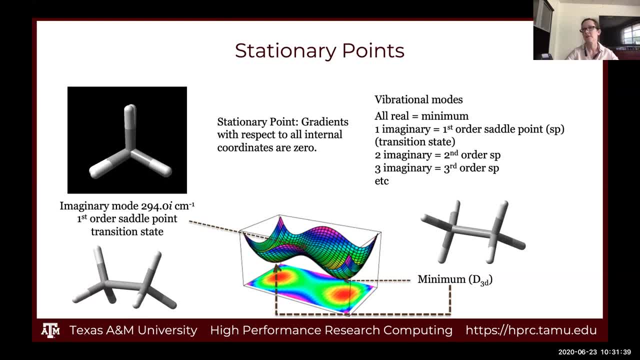 but very important to the research that you're doing. Okay, just like, if you're doing something experimental and you get odd results or results that you weren't expecting, you should think about. you should think about what those results mean, because they may be very important to the research. 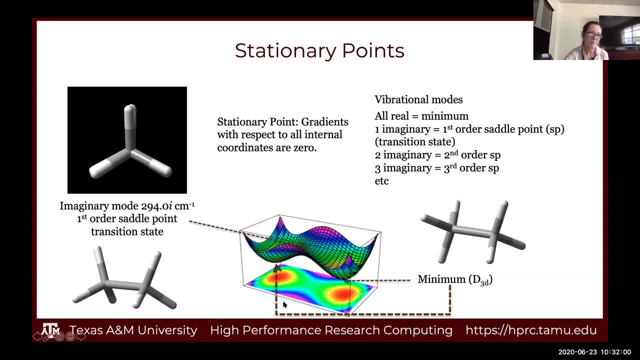 that you're trying to perform. Okay, so this is a first-order saddle point, right? so here's the person sitting on the saddle. That's why they call it a saddle point, because it looks like a saddle. And then here's the another person sitting on the saddle, and they're 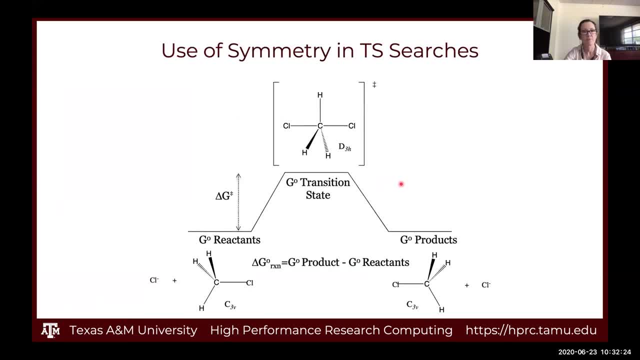 an edge point. You're looking at the foot, So just looking at both sides of the saddle and the foot. So you want to be an edge point. you want to be an edge point. at least there's no edge point. So I'm going to take my wrong side and go. I'm. 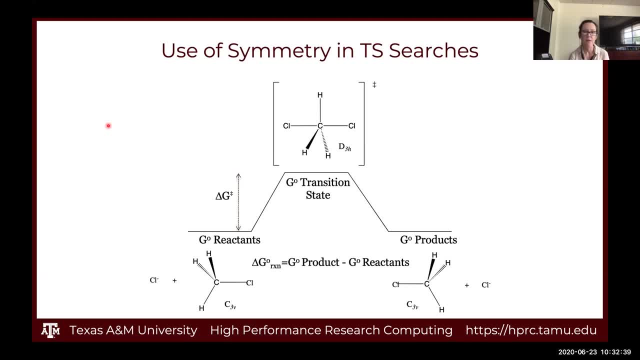 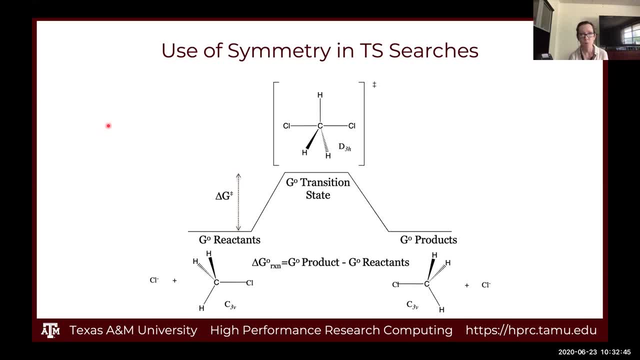 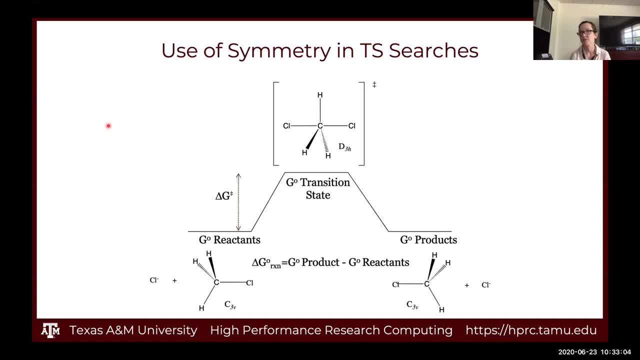 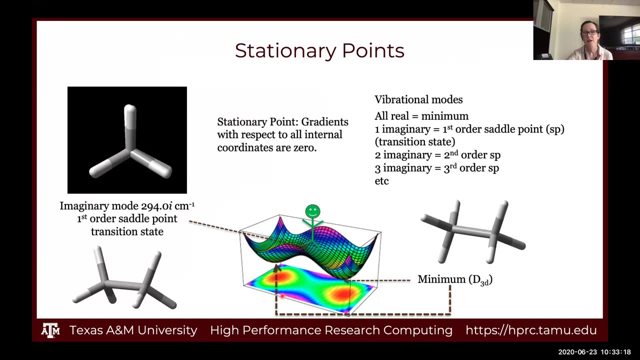 it makes it a lot easier to calculate transition states on the reaction chemistry. So there was a question on the previous slide as to what these coordinates mean. So there's really no. this would usually be some kind of a coordinate like a bond distance or an angle. okay, 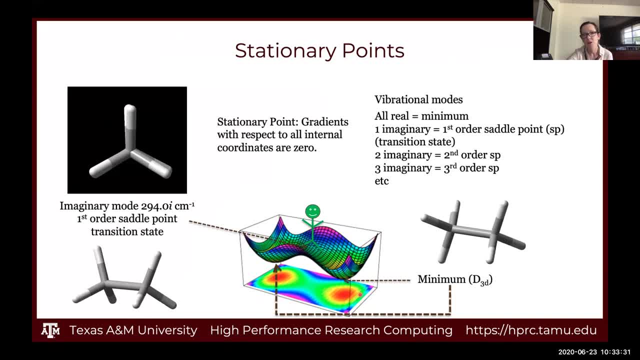 Two different maybe coordinates on this one bond or angle, two bonds, something along those lines. This one here would be energy. So this is definitely energy. So I should label that one energy, but this is a fictitious, you know. 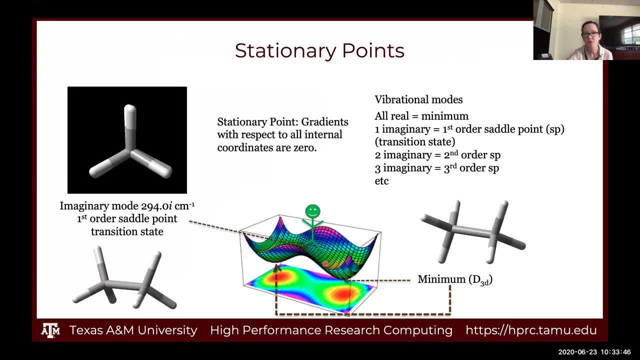 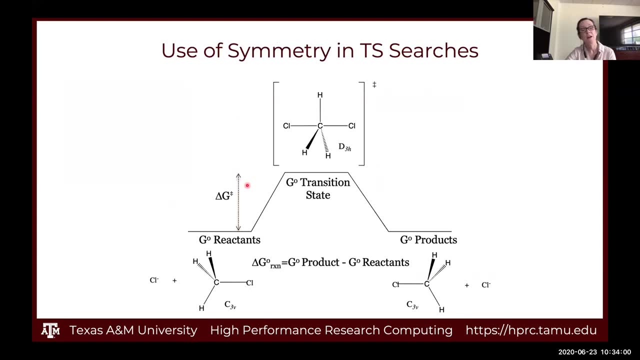 two coordinates that would be consistent with this change in reaction. okay, So this is a schematic. Okay, so, as I mentioned, it could be very beneficial to have symmetry to find transition states if the point group changes. So this is just a standard SN2.. 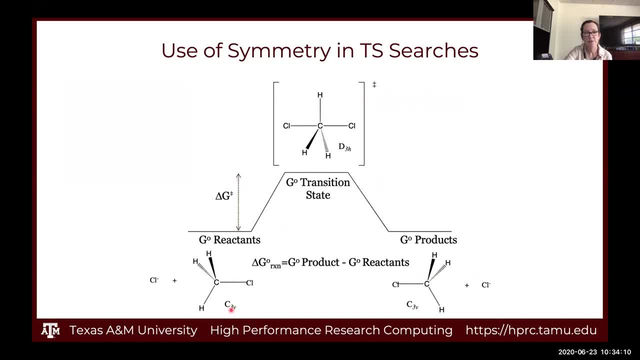 So here we have C3V symmetry, We have three planes of symmetry, We have multiple rotation axes. So, like I said, if you're not familiar with point groups and symmetry, that one webpage that I listed is a really nice tutorial. You'll probably want to go look at that. 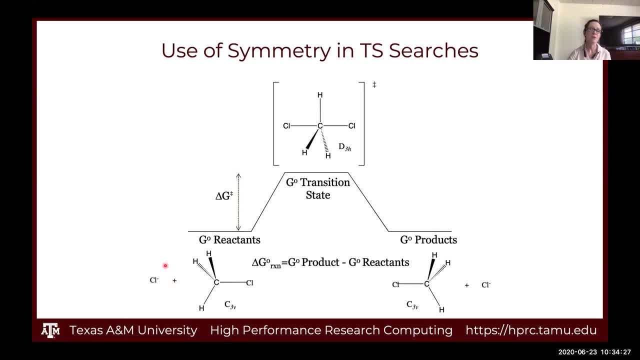 if you're going to be doing calculations with molecules that have symmetry in them. So if you have a difference, then you can just do a standard geometry optimization on your reactant and C3V symmetry And then you can do a standard geometry optimization. 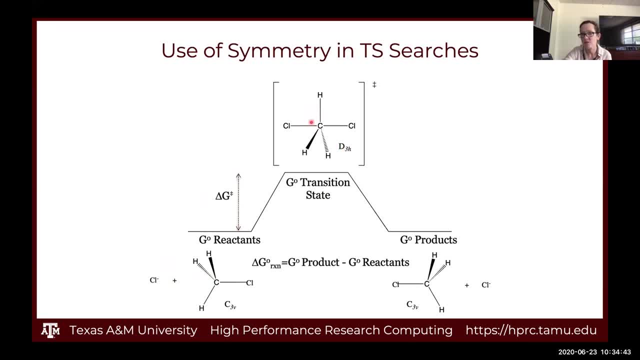 in D3H for the transition state that is shown here. okay, So the wedges here, this is coming out of the plane And this is going back into the plane. okay, Coming forward, going back, And then these are in the plane. 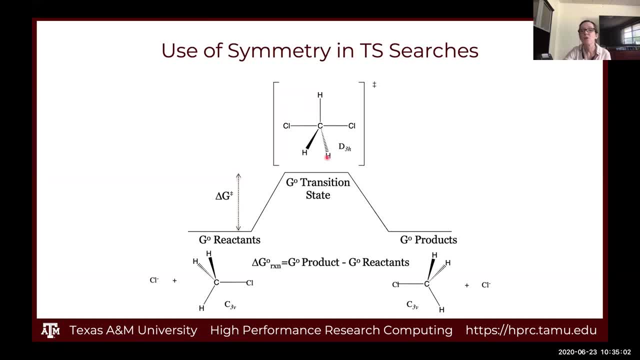 since there's no wedge on it. So for D3H symmetry, this is a minimum, But in C3V it's a transition state okay. Or in no symmetry it's a transition state okay. So that's why you can do a standard geometry optimization. 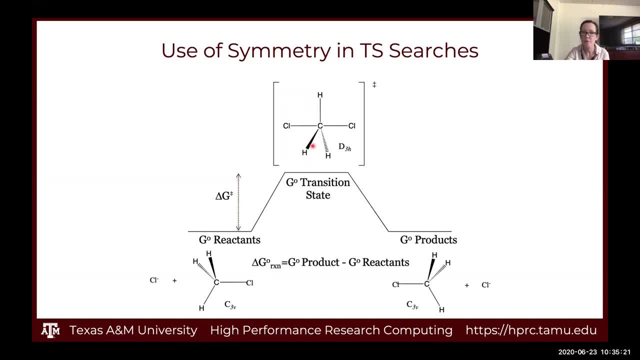 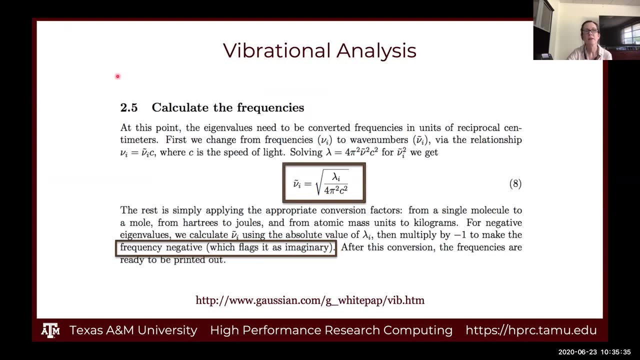 It makes it a lot easier to find these transition states And we are going to be doing, during the hands-on sessions, calculations for optimizing to transition states. Okay, so we've talked a little bit about geometry optimization And we talked a little bit about frequency calculations. 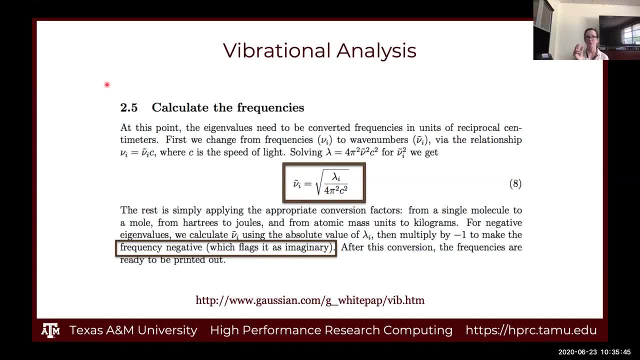 The frequency calculations calculate those vibrational modes. okay, And I showed you the vibrational mode for the imaginary mode of the ethane twisting right At the transition state. So eclipsed ethane, the imaginary mode was a twisting motion about the carbon-carbon bond. 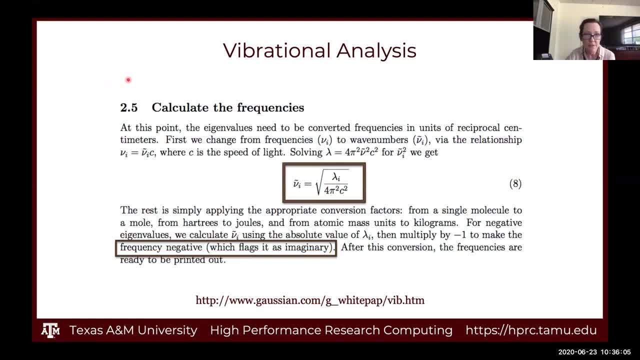 So one of the things that was listed there was that it was an imaginary. it was an imaginary frequency. In most programs, when you have an imaginary frequency, it puts a negative sign in front of it which flags it as imaginary. The reason it's an imaginary mode is the frequency. 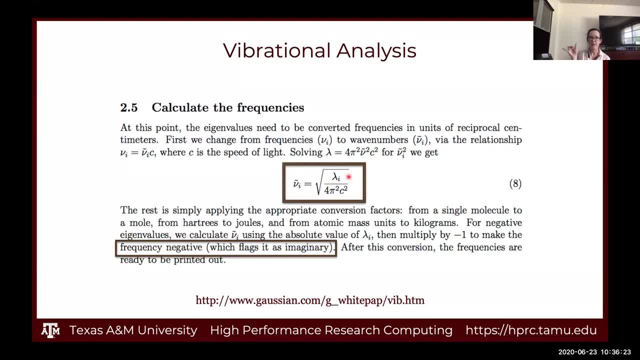 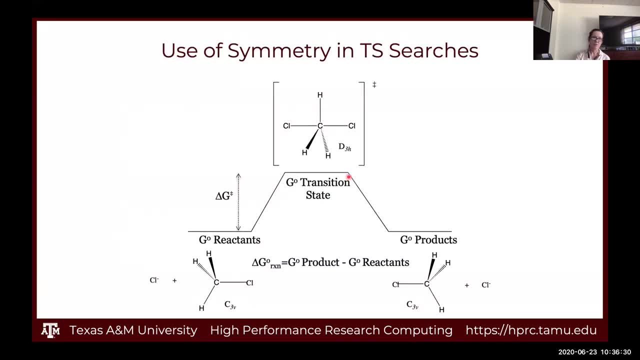 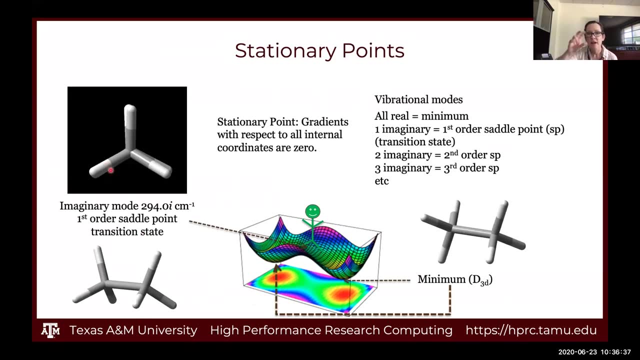 is the change in the energy, okay, Divided by some constant and taking the square root of it. At that point, right here, okay, At the transition state, Okay, This vibrational mode will take it down in energy, right, So at that mode it's going to take it down in energy. 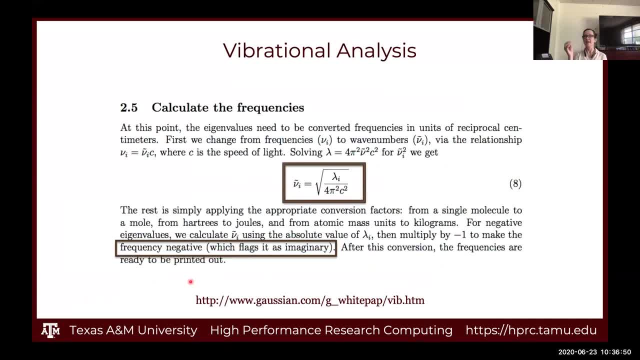 which means that the difference in energy at that transition state for that vibrational mode is negative. And if you take the square root of a negative number you get an imaginary mode. So that's why in first-order transition state theory the transition state has one imaginary mode. 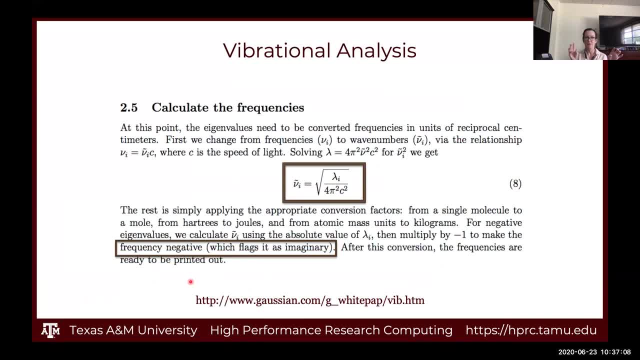 It's one vibration That takes it down in energy, that connects the two minima on either side of it. okay, So when you read in the literature that the transition state has one imaginary mode or the reactant has all real frequencies, that's what they're talking about. 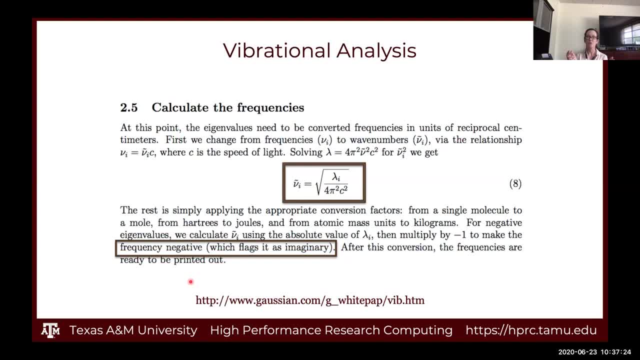 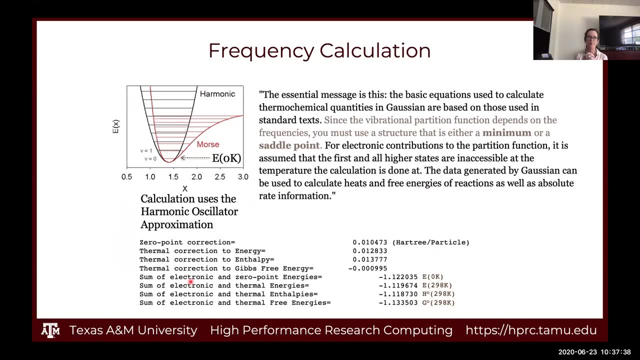 That's how you characterize whether or not it's a minimum on the energy surface or a first-order subtle plane which is a transition state. Okay, For the vast majority of these quantum calculations, molecular systems, the frequency calculation is using an harmonic approximation. okay. 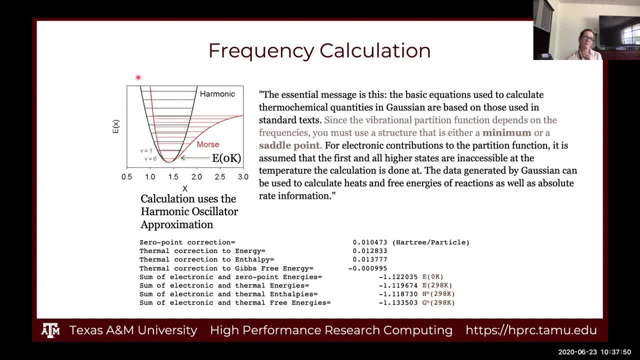 So the harmonic approximation which is shown here, it's to first order. In reality, the vibrational well for molecules is more Morse-like, okay, Where you have something that is asymmetric. So what this means for your calculation is the higher you go in the vibrations. 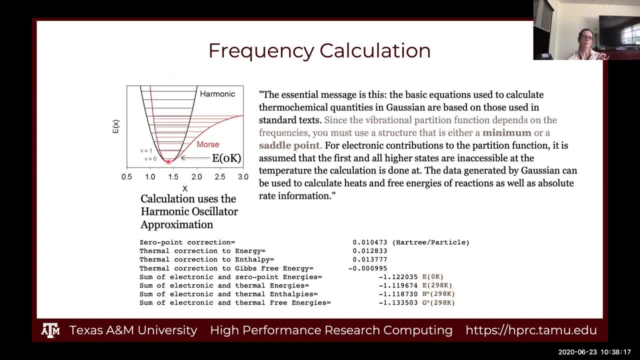 the larger the error will be okay. So as you move up in the vibrations, the error will get larger and larger, Okay. so what I also want to point out here is when you're doing a geometry optimization, you're calculating the energy. 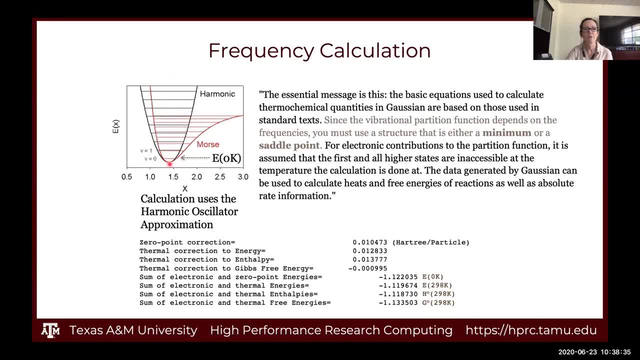 all the way at the bottom of this. well, So you have not included even- it's not even- the energy at zero k. You're all the way below zero k. It's a non-realistic number. okay, This is the electronic energy for the system. 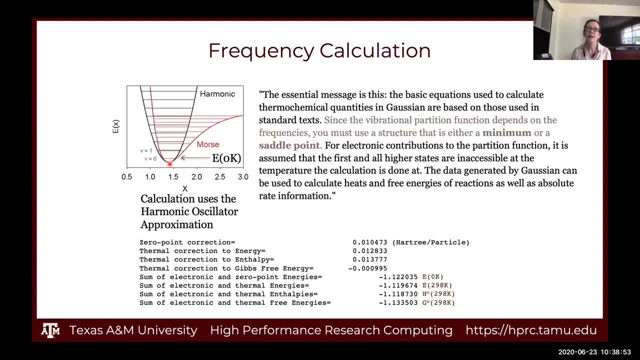 It's not even the energy at zero k. To get the energy at zero k, you need to do a frequency calculation, because you need to get the first vibrational level And that will get you the energy at zero k, Okay, And then it can also populate the vibrational levels. 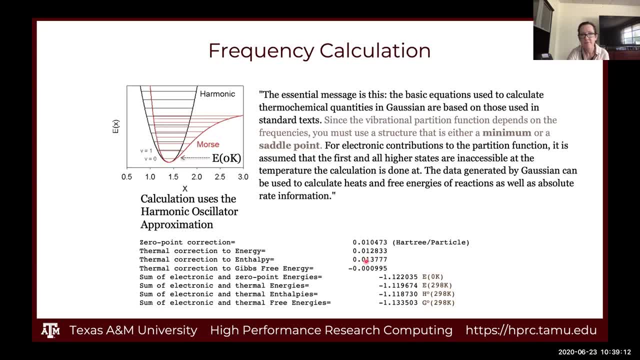 So you can get the thermal corrections that you can get up to the enthalpy. Okay, you can get the energy at 298 and the enthalpy under standard conditions and then the free energy under standard conditions. But if you do a standard geometry optimization, 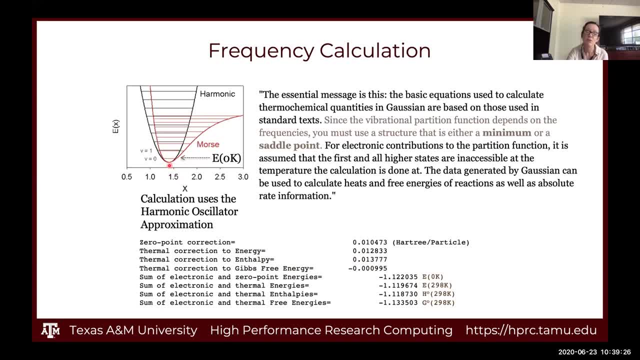 you're only getting the electronic energy Optimizes on the electronic energy surface And that is a consequence of the Warren-Oppenheimer approximation. So frequency calculation that's required to get the energy at zero k, the energy at the first vibrational level. okay, 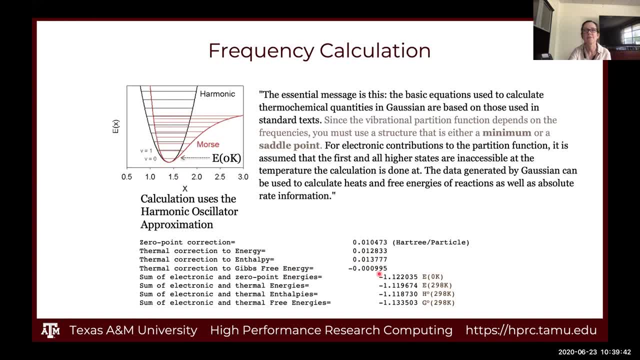 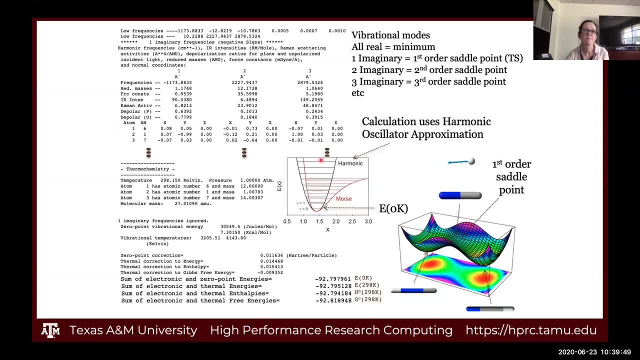 And the enthalpy and free energy under standard conditions. Okay, so here's a standard output from a Gaussian calculation and the information it'll provide. So this is for HCN. We have the reactant, We have the product And this is our transition stage. 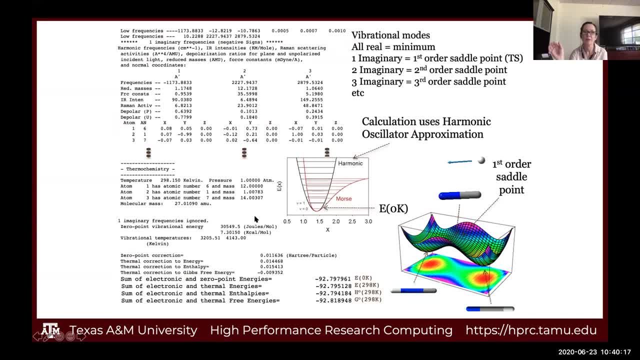 Where you have the hydrogen moving back and forth between the carbon and the nitrogen. So this is our first order saddle point. Okay, now remember, this is within the harmonic approximation. It lists all of the frequencies. So it lists all the frequencies. Here is our imaginary mode. 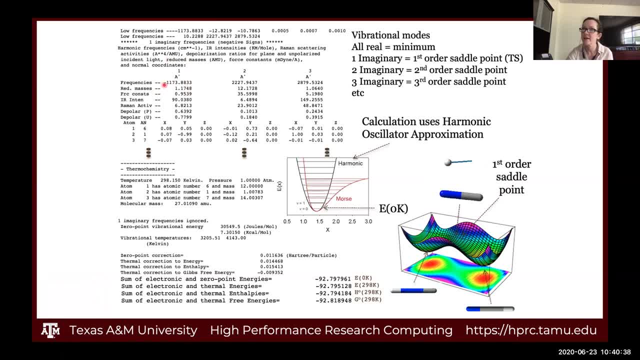 Okay, the first vibration should be tagged with a minus sign, so that we have an imaginary mode. And then all of the other frequencies going up are real. They don't have the minus sign on them. Okay, and you can look at all of these different frequencies. 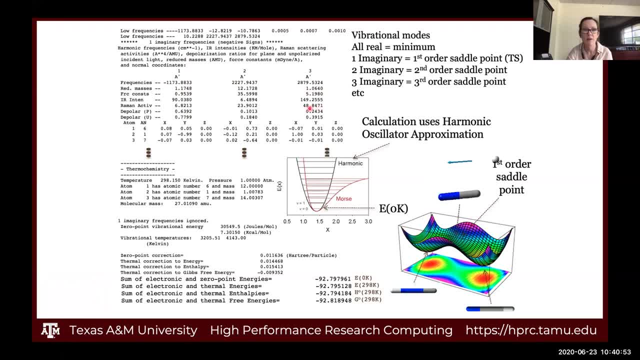 and see what kind of mode they have. So this is just a three atom molecule, So we have very few frequencies here, And then down here it will actually give you the oops. sorry, It will give you the I'm energy, is there okay? 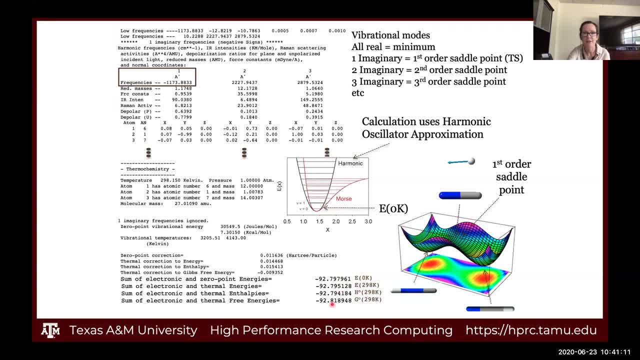 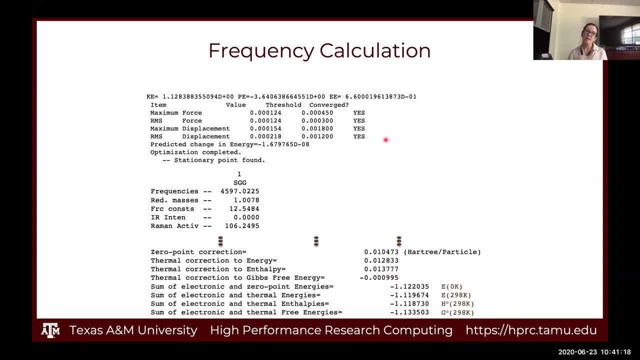 The enthalpy under standard conditions and the free energy under standard conditions. Okay, so when it does a geometry optimization? I'm not sure if you remember, but we had two iterative processes. Okay, we had a wave function iteration- Okay, to optimize the wave function. 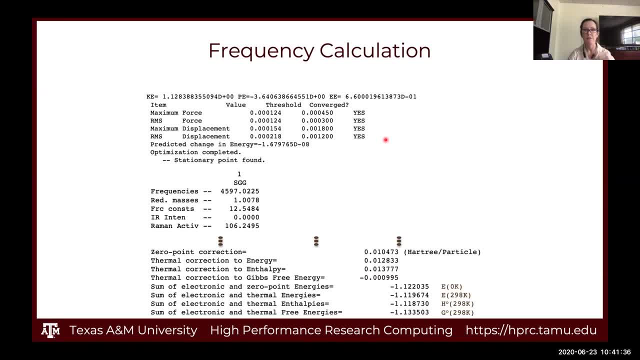 And then we also had a geometry optimization. So we had to do a geometry optimization iterative process and these are both self consistent. It looks at the last step and compares it and decides whether or not it's converged. So if you do a geometry optimization, 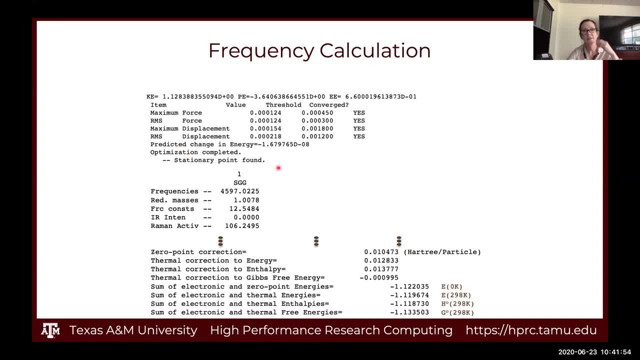 and then a frequency calculation. it's going to give you a listing of maximum force- root mean square in force, maximum displacement and root mean square in displacement, And this is in regards to the phase in which this motion happens. Okay, so now you have a geometry optimization iterative process. 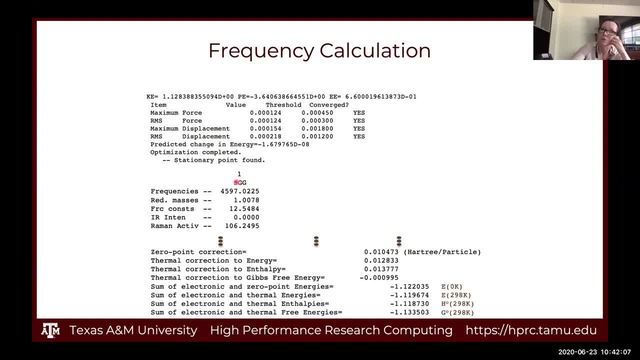 the movement of the atoms from one geometry step to another and the forces on it. So there is a value that it's achieved, and then there's a threshold and then it's whether or not you've achieved that, falling under that threshold that is imposed If you get all four yeses. 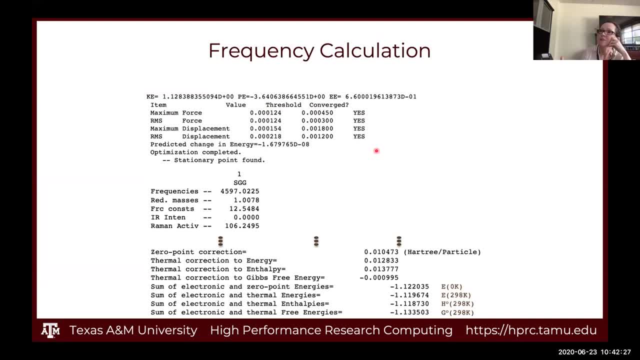 that means that it thinks that it has reached the bottom of the well for a minimum, or the top of the point for a first order. saddle point: If you don't have all four yeses, it's actually not uncommon, if you have a very flexible molecule, that your forces converge. 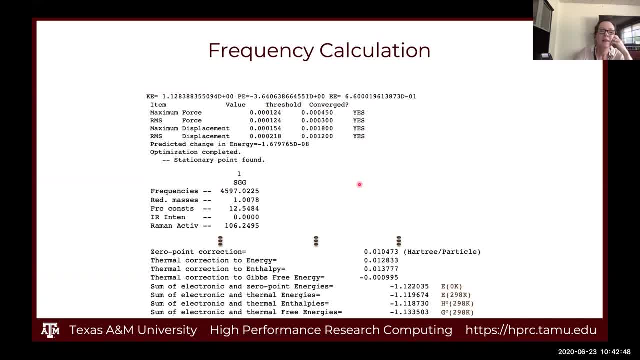 but your displacement does not- And that is a consequence of a very, very small force- can cause a large displacement. So you want to see four yeses, but it's not uncommon To get two nos and two yeses. It will tell you if it's reached the optimization. 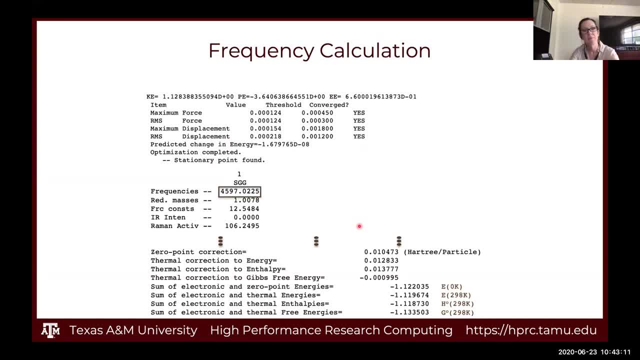 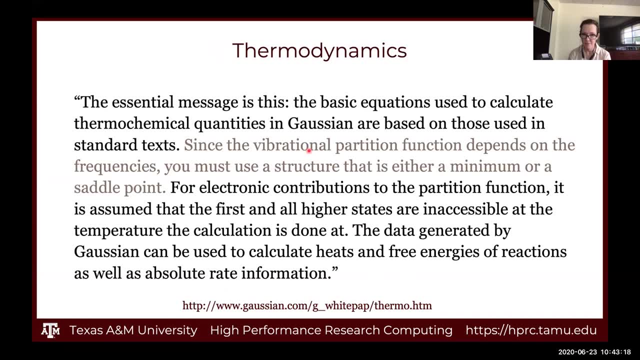 give you the frequencies and, of course, the energies. Okay, A little bit about the energies, the thermodynamics. One of the consequences of using the harmonic approximation to first order- the harmonic approximation to first order right- is that you need to be at a stationary point to get good thermodynamics If you're not at a stationary. 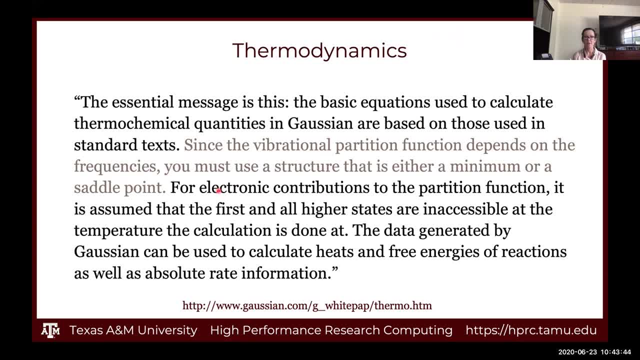 point. if you're not at a minimum or a first order saddle point, the potential well is very anharmonic and your thermodynamics are not going to be accurate. Okay, So when you're looking at energetics from these molecular calculations using quantum mechanics, you need to take them at the stationary. 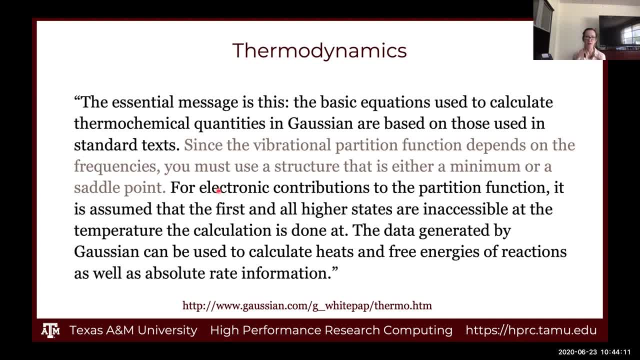 points, Otherwise you're going to get anomalies and poor quality results. Okay, So if you want to learn more about the thermodynamics from these calculations, there's a white paper on Gaussian's webpage that you can go through. Okay, And it's just emphasizing that the structure needs to be a. 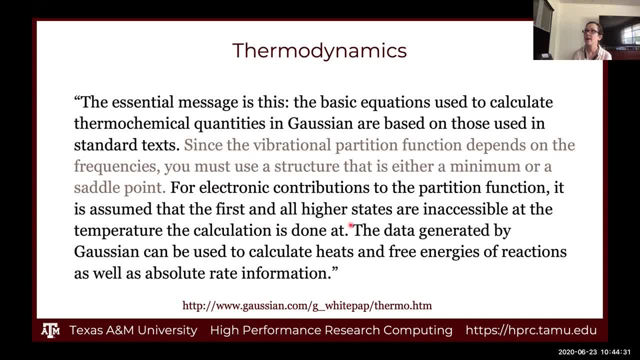 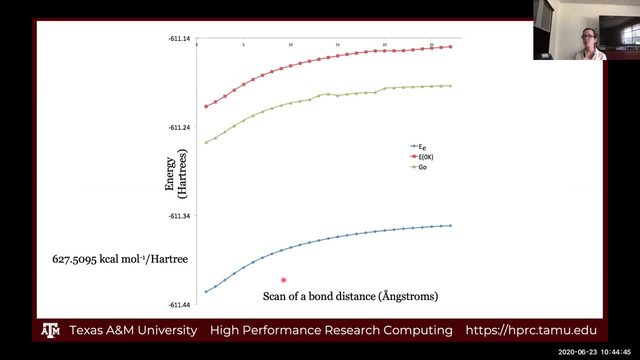 minimum or a saddle point, Okay, And that's because we're only looking at the harmonic term. So here is just an illustration. If you're looking at scanning a bond distance, Okay, So we're no longer at the minimum or the transition state. 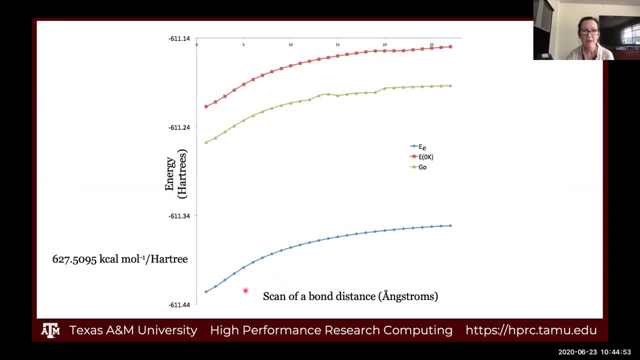 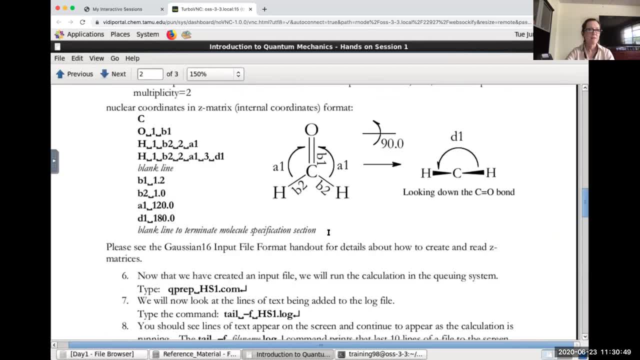 Okay, Remember, the electronic energy is all the way in the transition state. Okay, So we start here and this is the electronic energy is nice and smooth. Okay, So at this point I want to go ahead and stop recording And I want everyone to try to. 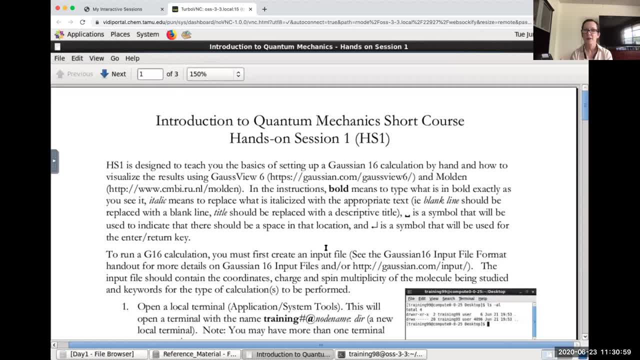 walk through this hands-on session, Okay, And if you run into problems, then I want you to put information in chat. You can either send it directly to me or you can pose the questions to everyone. Okay, And then at 1150, I'm going to go ahead and walk through. 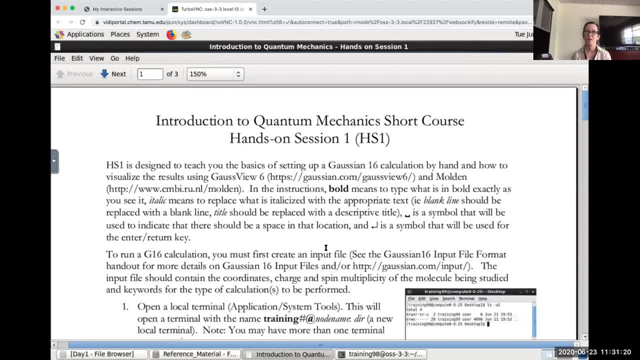 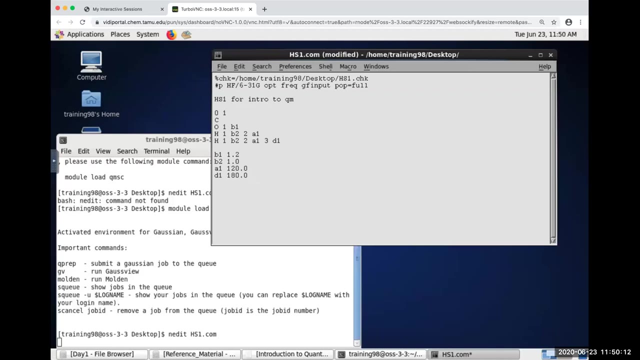 all of the steps that I just talked about, to show you what it should look like. Okay, Okay, So some of you may have gotten through a fair bit. I'm setting up submitting calculations. Some of you may have gotten stuck. That's okay. Right now, what we're going to do is I just want 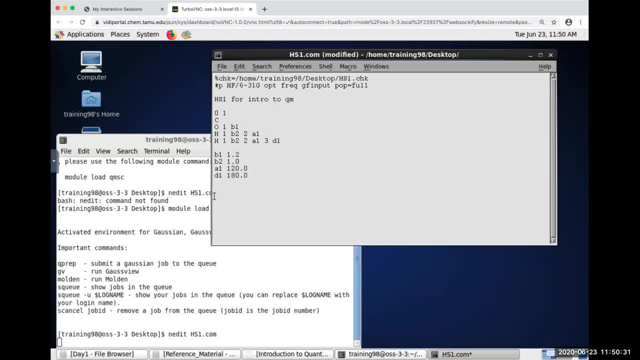 to go through the steps that I verbally walked you through earlier, And then you can continue to work on this or we can revisit it during the afternoon session. Okay, Okay, So I've typed in the input file that I gave you in the hands-on session one. 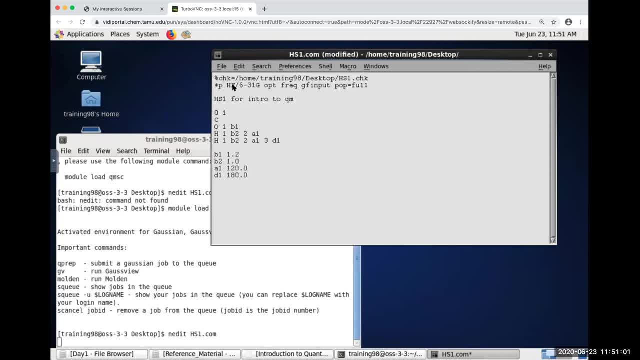 tutorial. So I have my percent check line. You'll notice that I have these. you know the spaces and the blank lines instead of the special characters. And then one thing I want to point out is that is not a blank At the end. So if your cursor ends here and there's nothing else below it, that's not a 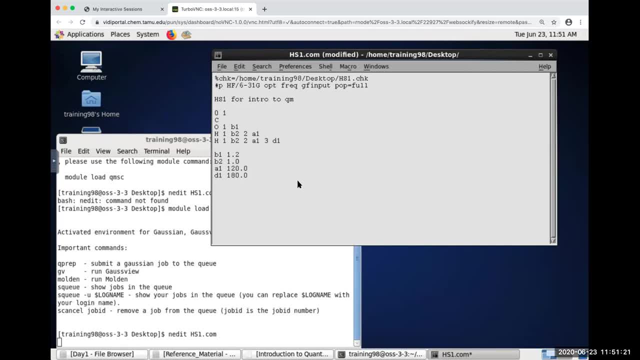 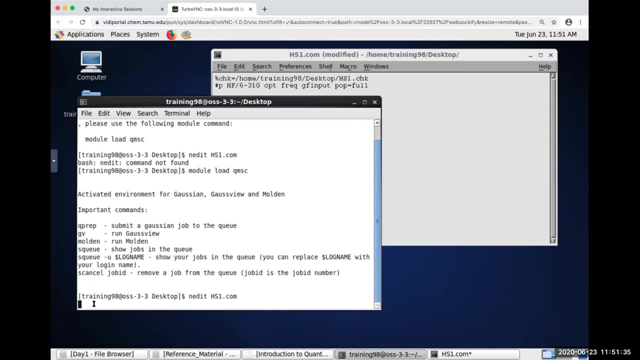 blank line. That is a blank line. Okay, It needs the enter at the end. Okay, So I have my file now. The other thing I want to point out is, if you'll notice, here at my prompt I've got my N edit here and my cursors down here If I try to type in a command here. 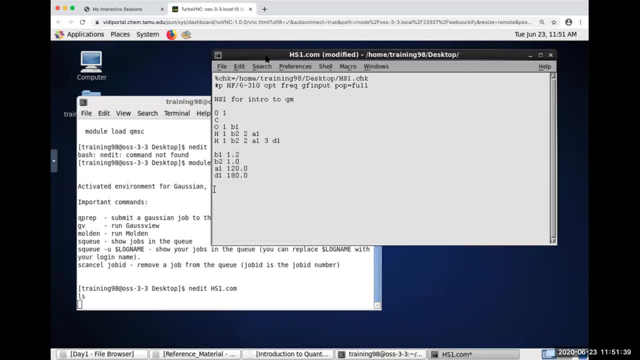 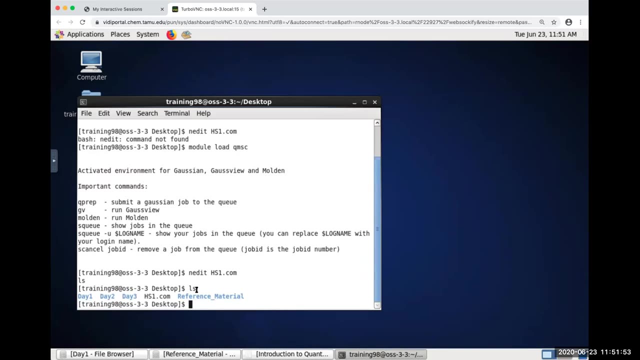 nothing's going to happen And that's because N edit is running interactively. For me to get my prompt back, I have to close and edit. Okay, So I'm going to save my file and I'm going to exit And you'll notice that it caught up with my command. Okay, So if you type in a command at 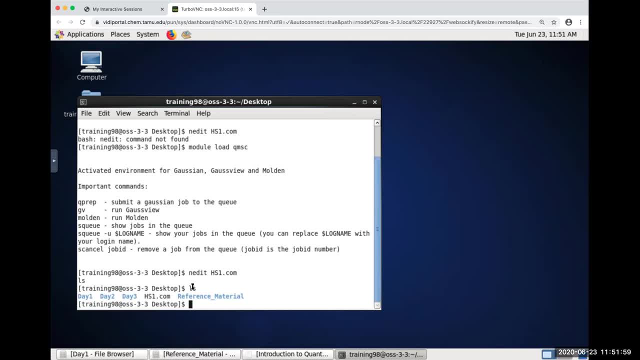 the prompt and it doesn't respond. don't keep typing in commands. Try to figure out why it's not responding before you keep typing in commands, because it'll try to catch up if it can. Okay, So I now have my file here. Okay, Now one thing you might notice. 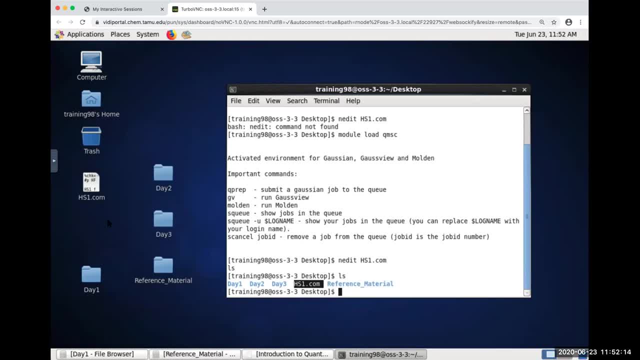 is. sometimes files will appear here automatically and sometimes they won't. Okay, So don't be surprised if you've created a file on your desktop and it doesn't automatically appear. Sometimes they won't with the graphical, but you can always see them. command line with the LS. 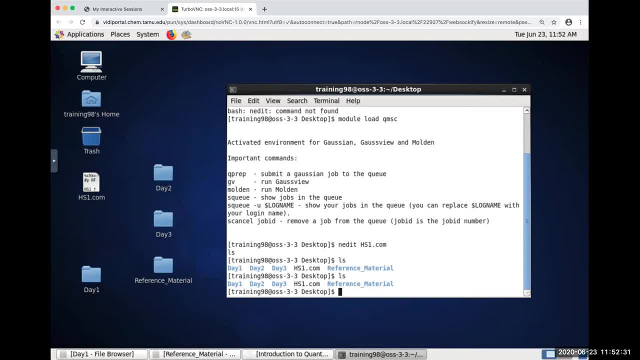 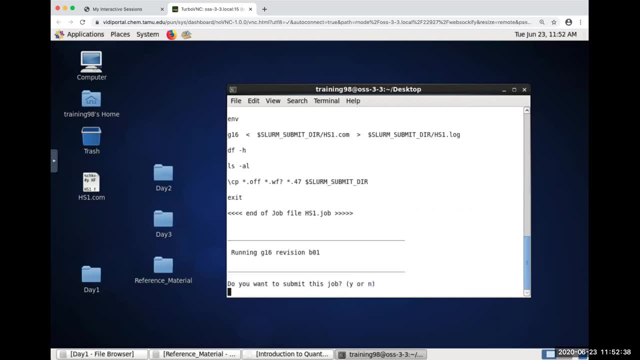 Okay. So I type LS to list my files. There's my hs1.com And now I'm going to go ahead and submit that to the queuing system. So I type Q- prep my file name. It says: do I want to submit? 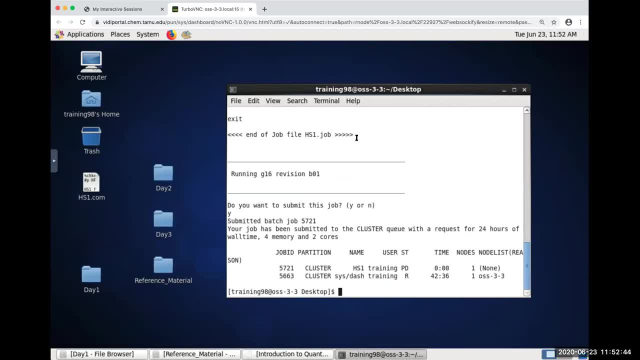 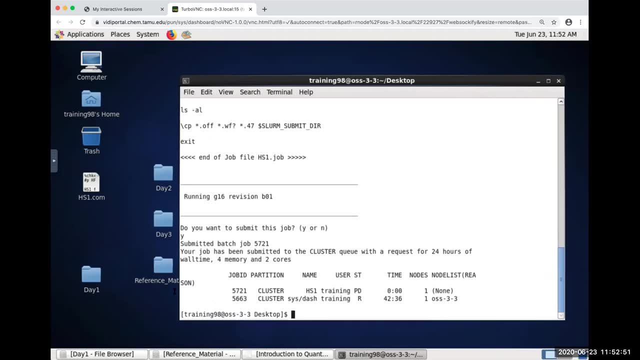 it? Yes, I do, And now I've submitted the job, Okay, And it shows my jobs that are running in the queuing system. So I have two of them. One of them is my dashboard. Okay, Make this lease. Okay. 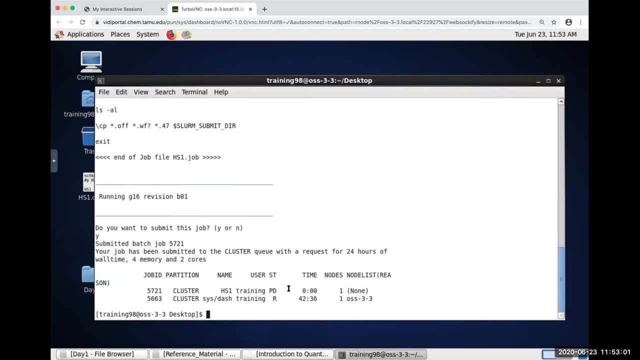 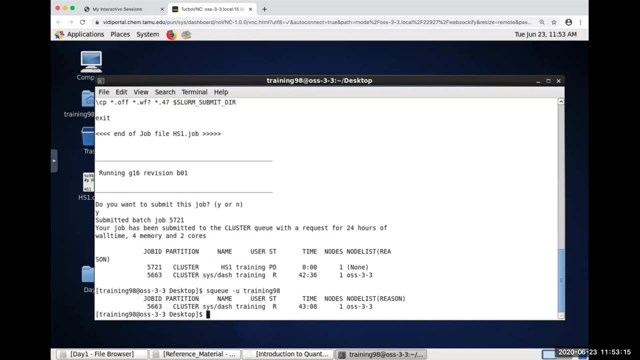 So one of them is my dashboard with the open on-demand portal, And the other one is my job, going to be running in the queue Right now. it says that it's waiting, Okay. So if I type SQ, dash U and my username, Okay, It'll update the information. Now my job is already out of the 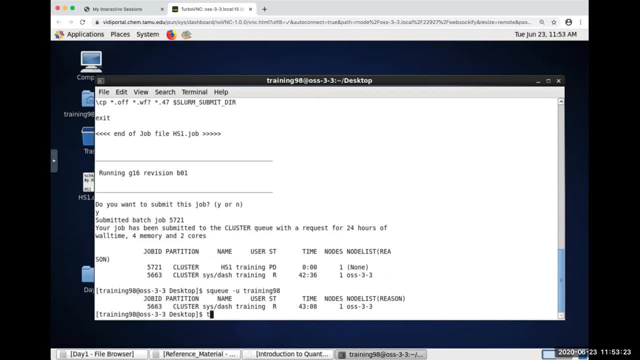 queue. Okay, It's no longer listed. I only have my dashboard. but just to show you what it looks like, do tail dash F and then my output file. So the input file was hs1.com, Right, And then I also mentioned something about an hs1.chk. That's the binary output. 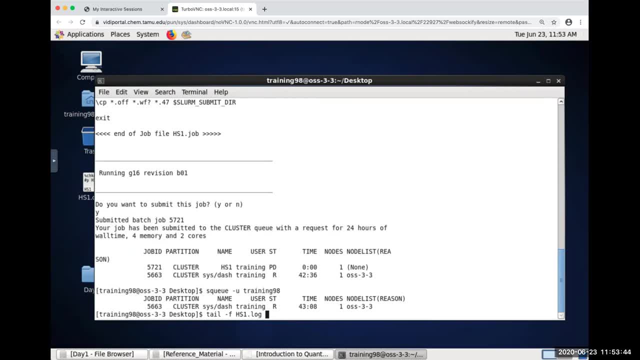 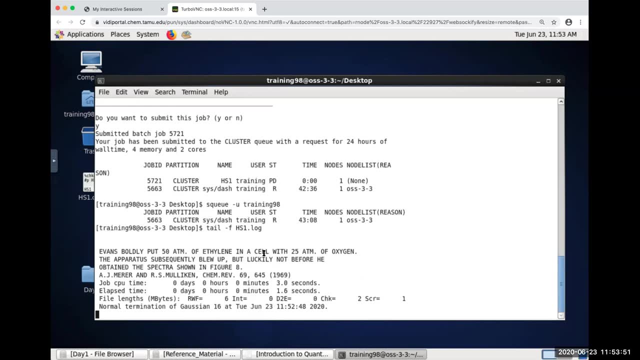 File. Okay, That the program reads. And then the human readable one is the hs1.log. Okay, So if the calculation was still running, more information would be popping up as it was running. Okay, But right now, since the calculation is not running, all I see is the end. 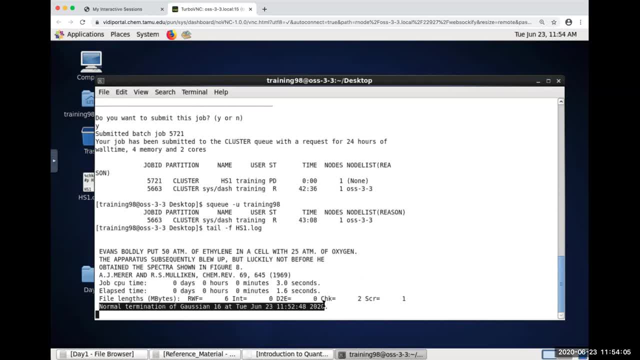 which is the normal termination of Gaussian 16.. Okay, So this is a good sign. This means Gaussian thinks that it's finished. normally That doesn't mean you got the right answer Or that you got what you were expecting. That just means Gaussian thinks that it finished. 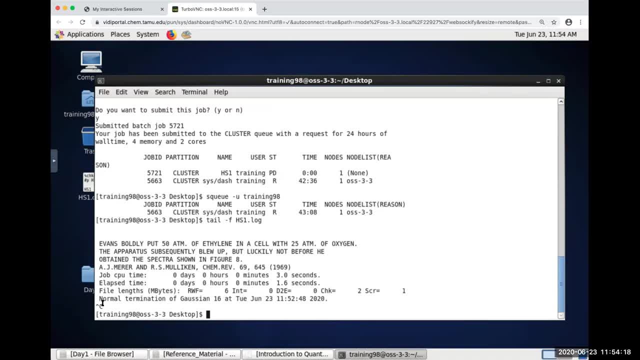 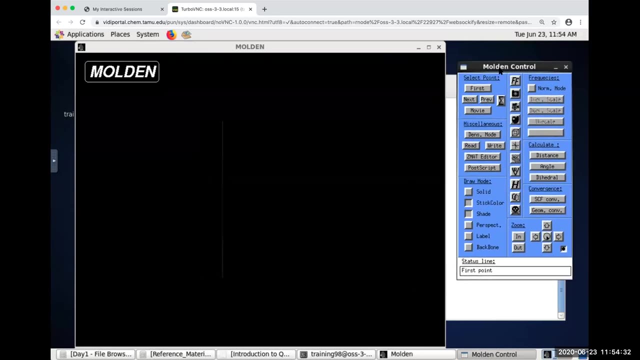 normally. So I'm going to type control C. You'll notice that it shows up here. Okay, So it brings me back to my prompt. All right, So now I'm going to use Molden to look at this result. So Molden is a little bit clunky, but it has a lot of unique features that are quite useful. 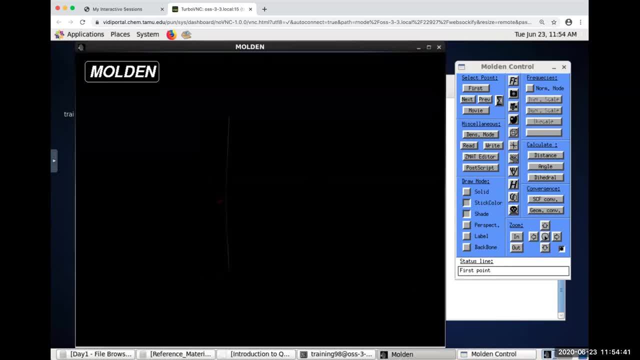 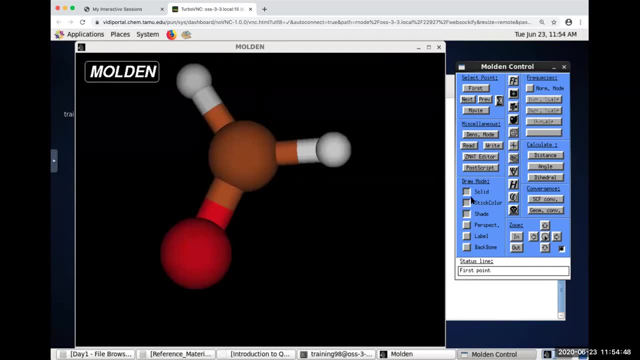 So here's the control panel. Looks like I don't have a molecule but I do, And that's just because it was looking straight down and it was on stick. So if I change it to solid you can see it better. I'm going to click. 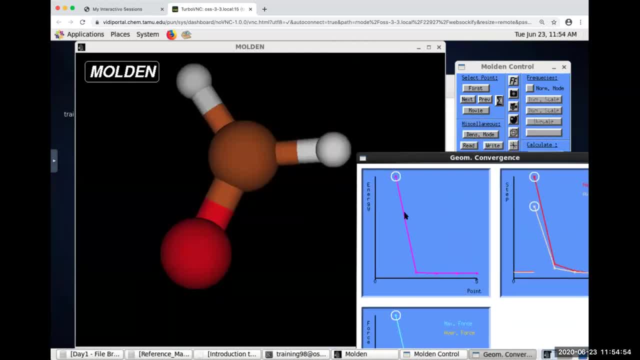 Geom Convert. What this is showing me is the energy change at each geometry optimization step. So here's my first one. You'll notice it starts with the starting structure, The second one and the change in energy in Hartrees. Okay, So there's a big change in. 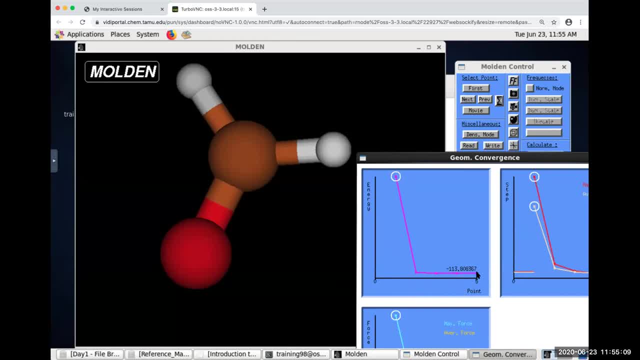 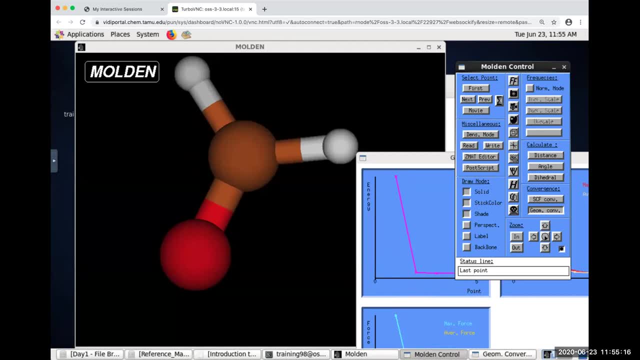 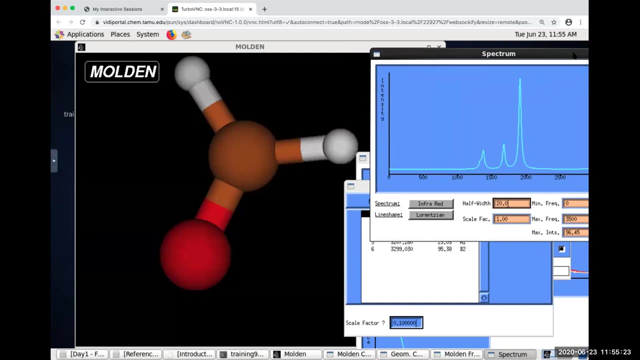 energy and then it levels off. It took five geometry optimization steps to finish And then I can also click movie and it will show me the change in the geometry, which was not substantial, Okay, Okay, So you can also look at the normal modes. Here's my spectra, right, I can click on. 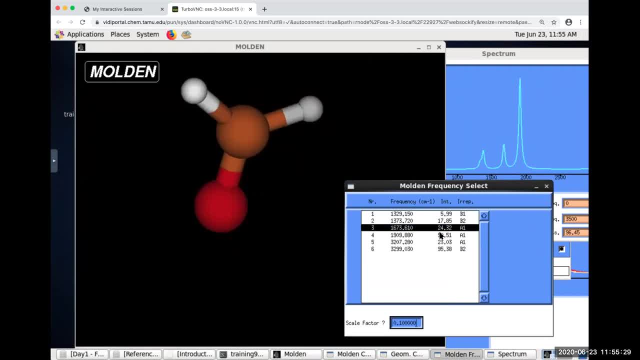 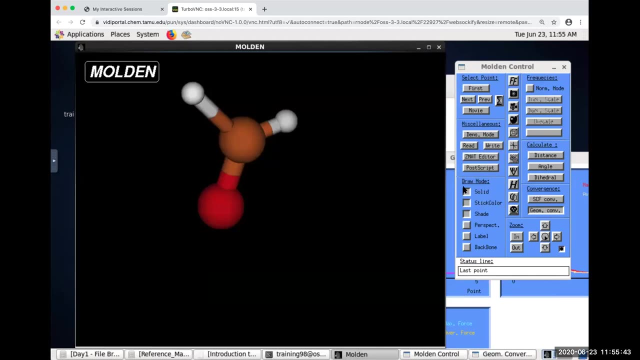 the different vibrational modes and it will tell me, or show me, what they look like. Okay, And you can change the scaling factor to make them bigger. I can close that And that. Okay, I'm going to go ahead and put it back to the stick for a moment. 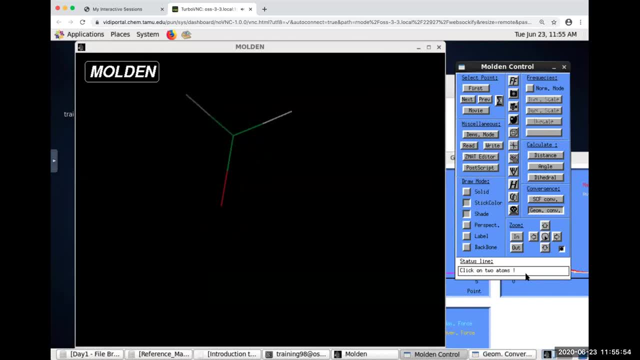 To do the distance, you have to click on two atoms And it's very picky about where you click. Okay, So it says: click on two atoms. If you don't click right at the center of the element, it's not going to take it. Okay, So since I was able to click right on the center, 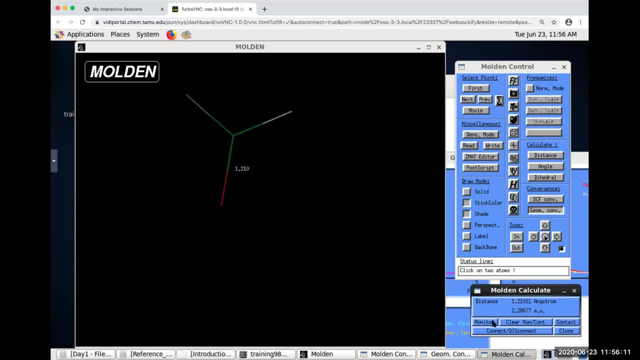 then this pops up. It gives me the distance and I can click on it. I'll click monitor and it will show up here. Now, if you click movie, it'll show you the change in the structure. Let me bring that back forward. 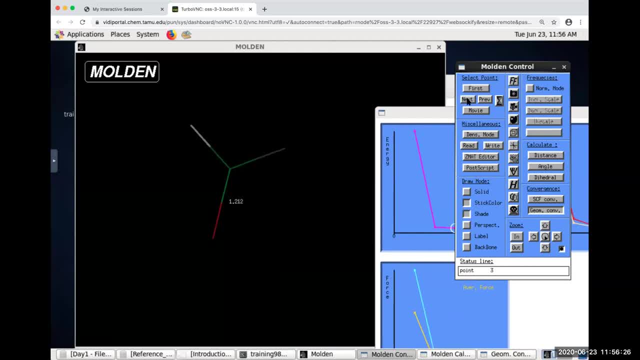 So if I go to the first point, it'll tell me the distance, And if I click next, it'll update the distance and how it changed when I was doing the optimization. Okay, So you can go ahead and play with different things in Molden. Now the way that you get out of Molden is: you can't close the window, It'll complain. It says: use the skull icon to quit molding. 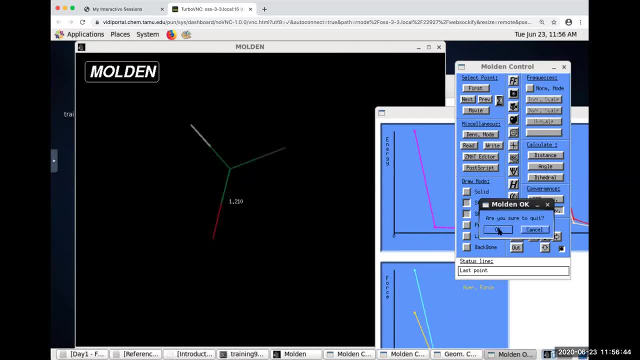 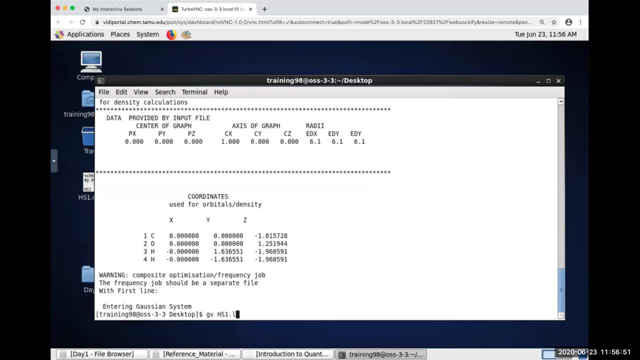 You have to use the little skull and crossbones right here And then you can click Molden. So now let's look at the results with GaussView. Now, this is one of the nice things that I like about Linux is, instead of having to load the program and then say file open, you can just usually say the program name. 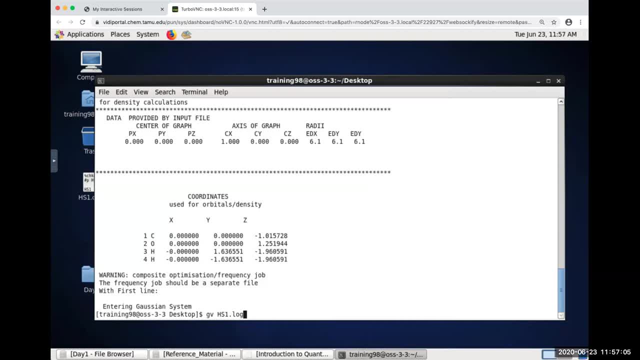 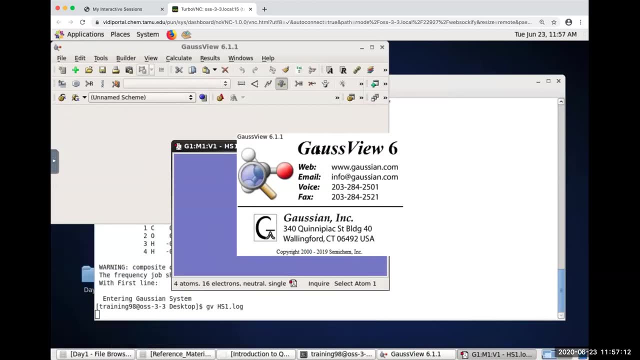 Okay, And then the file that you want to open, it will automatically open it. So you can just type GV, space capital, HS1 dot log and it will open the log file. You have to wait for this to go away, Alright. so here's my molecule Now. one of the main differences that you might notice right away is with Molden: it loads the starting structure, the structure that you drew and gave the program in the input file. 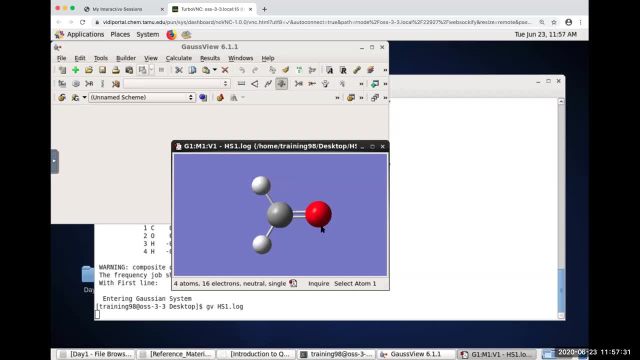 Okay, GaussView by default loads the final geometry and only the final geometry. Okay, so that's a major difference between the way GaussView and Molden works. It's a very important difference Because if you pull up Molden and you only look at the structure, it shows you that's the unoptimized geometry. It's the geometry that you provided, not the final result. GaussView shows you the final result if you load the log file. 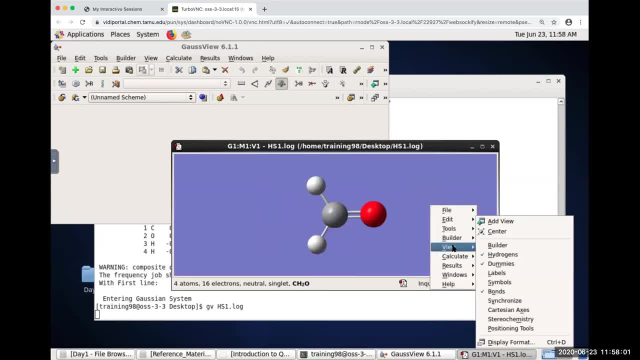 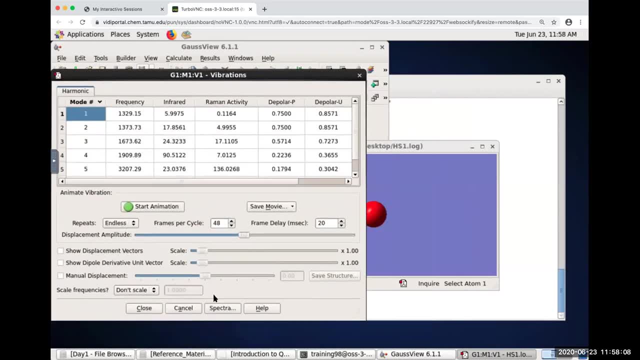 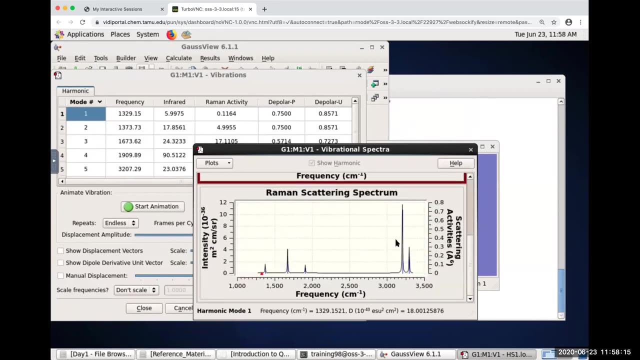 Okay, so you can also look at the vibrations in here under results and you can go to vibrations. Okay, if you want to see the spectra, you can pull up the spectra. It gives you the IR and in this case it gave us the Raman because we did a Hartree-Fock calculation. We'll go over that in one of the lectures. upcoming lectures. 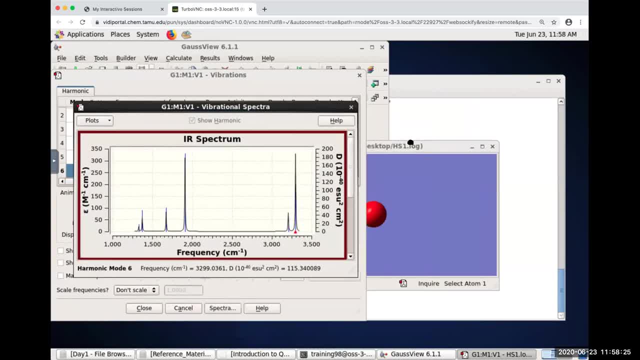 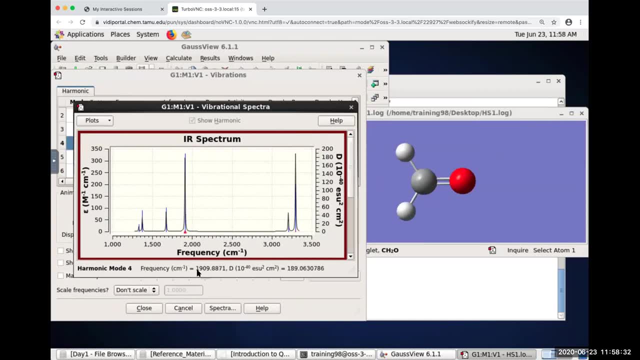 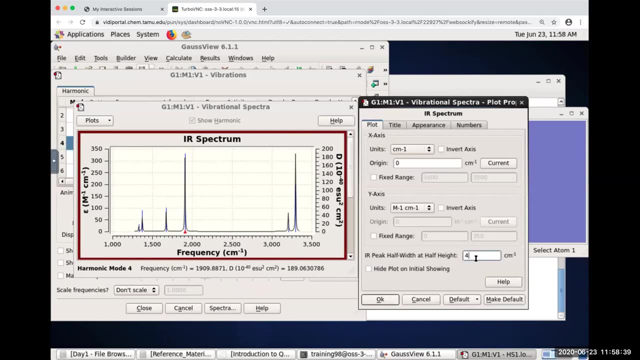 You can also click on the vibrations in here- Okay- to get the values on which one is which Okay, and their intensities Okay, and you can change the properties of this. So if you go to properties, you can change the, you can broaden it. 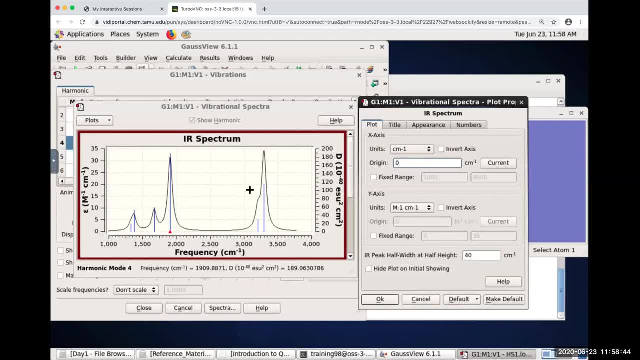 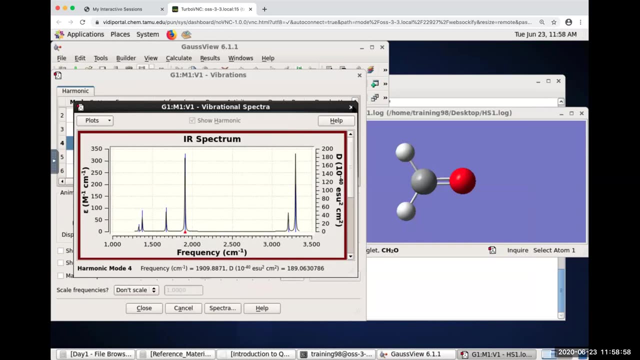 You can zoom in on parts. You can zoom in on parts, insert access, you can do titles and you can download this information So you can save the data and then import it into Excel. So there's lots of functionality in there. Like I said, this is licensed software, though You have to have a license for it. 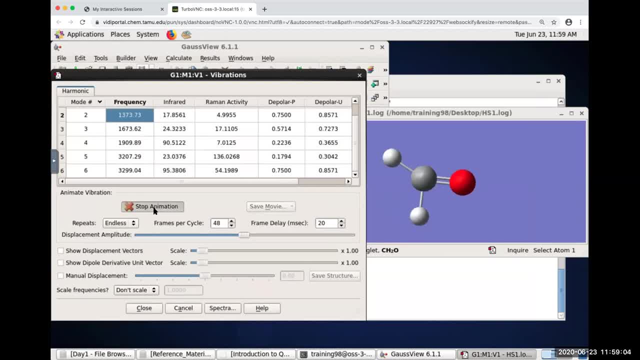 Okay, so if I want to see the vibrations, I just click start animation and it will show me the animations. I can also do show displacement vector. I can make this as a start. I can also do show displacement vector. I can make this as a start. 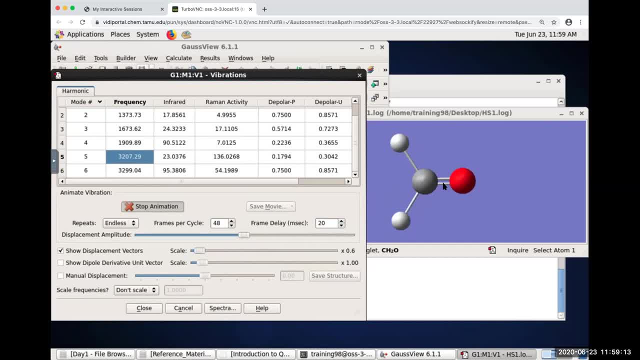 I can make this as a stop. I can make this as a stop bigger. make them smaller. okay, I'm not that one. you can change the displacement amplitude. you can make it really, really accentuated. kind of fun to watch. this is the best part of the calculations. 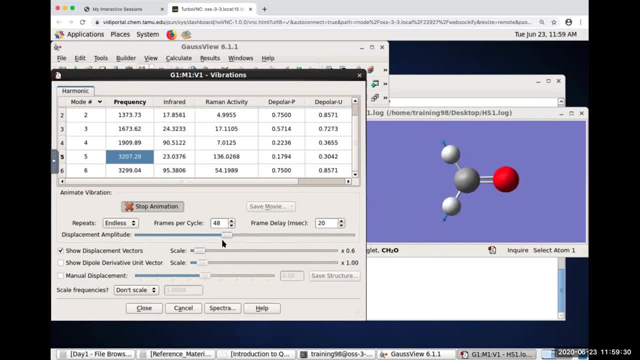 watching animations. okay, you can also do a manual displacement where you can push it along the vibration. now, the more accentuated you get- I am, they more- I'm forgot the way to say this- so the more you push it from its original structure at that vibration I'm, the less realistic the 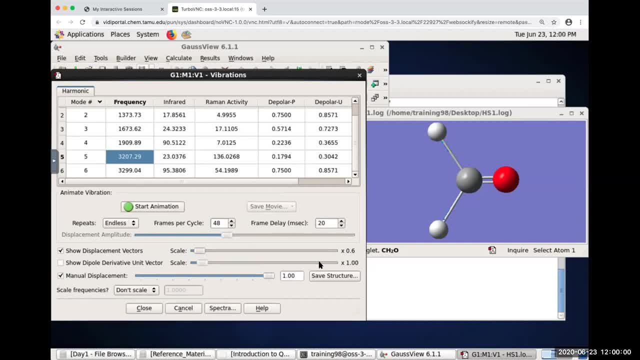 position of the atom is for the vibration. okay, so it helps our eye to be able to accentuate the vibrational mode so we can see what the motion is. I'm, but as you make the displacement bigger and bigger and bigger, the less realistic the location of the 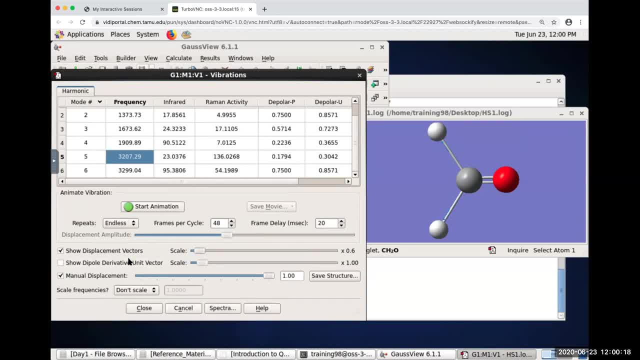 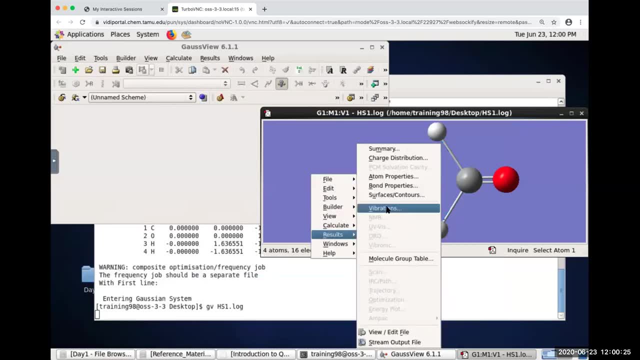 atom is okay, okay, so all right, it's enough for vibrations. oops, let me put it back to the way that it was. yes, good, okay, all right. if you want to view orbitals, they moved it. I always forget tools, so you go into the tools menu and molecular orbitals and 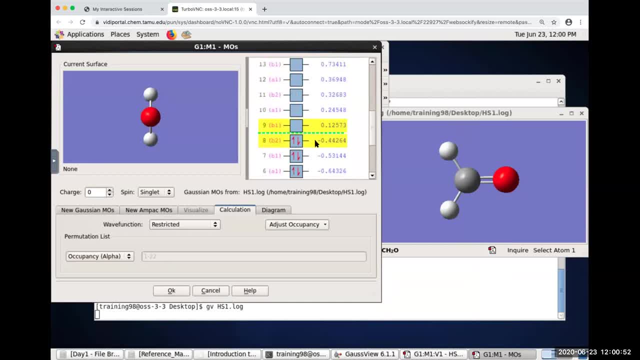 you get this not to scale molecular orbital diagram, okay, so this means there's two electrons in here. now, if you do this from the log file, your visualization tab is not available. okay, and that's because it requires the checkpoint file to visualize orbitals so you can see how much more. 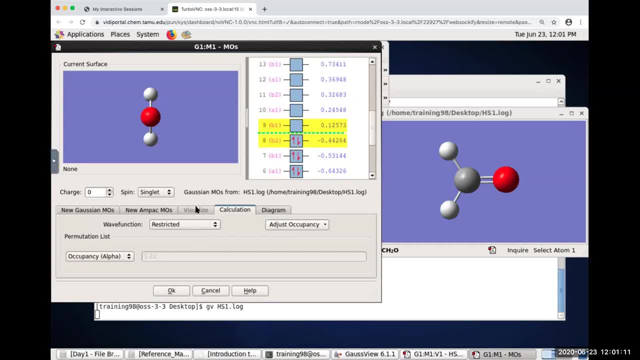 orbitals. So if you want to visualize orbitals you have to load the checkpoint file. You've already loaded the log file. As long as the checkpoint file is in the same place, it gives you the option. when you go to the new Gaussian MOs you can just click load okay, Or you can. 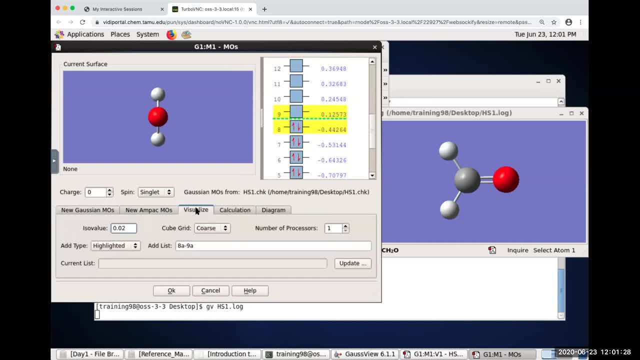 file. open and load the checkpoint file. Okay, now my visualize tab is available. This iso value is the value of the wave function that it's going to plot in space to make the surface okay, I generally like to use 0.04 or 0.05.. I'm going to go ahead and change it to 0.04.. So this is my. 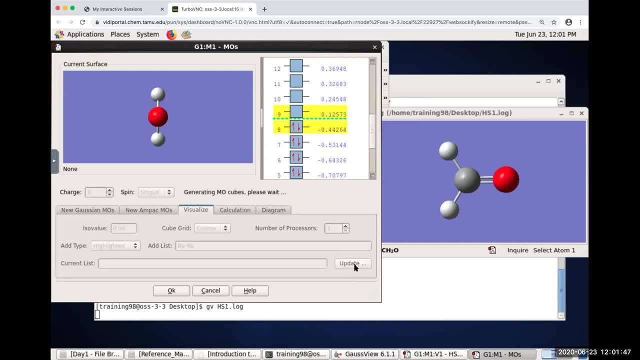 highest occupied molecular orbital and this is my lowest unoccupied. and I'm going to say update, Click on update. okay, And here are my molecular orbitals. So this is my unoccupied. There's no electrons in this one and this is my highest occupied molecular orbital, okay. 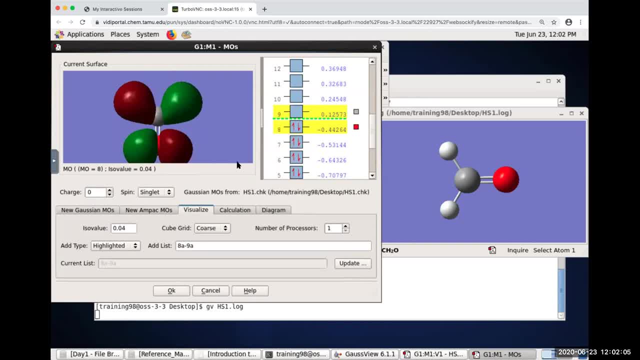 And you can right-click and change the way things view. I'll let you go ahead and play around with that. If you want to view more of them, you just have to highlight them and click update Now. historically, Gauss-Hugh has had a history of crashing while visualizing molecular orbitals. 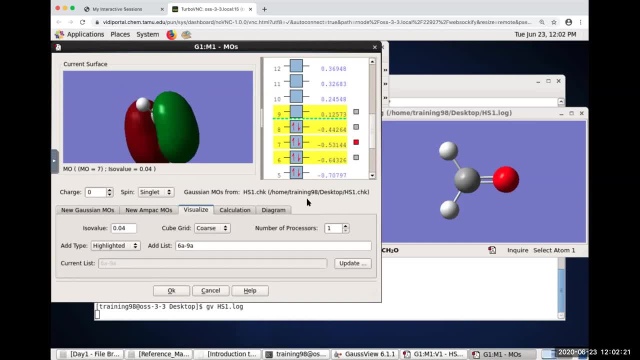 So if you plot a whole bunch of them, I would not try to touch it or do anything until this comes back, okay, Otherwise you increase your risk of it crashing, Okay. So that's why you can go through and look at your molecular orbitals. 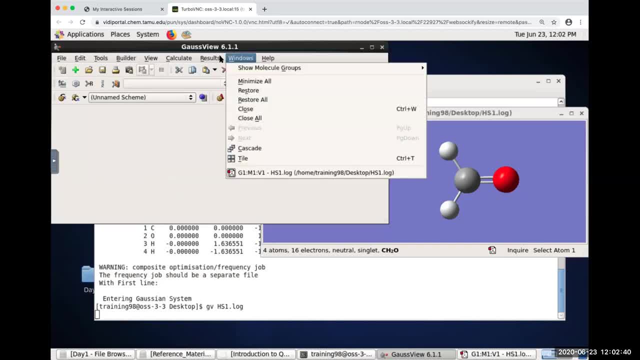 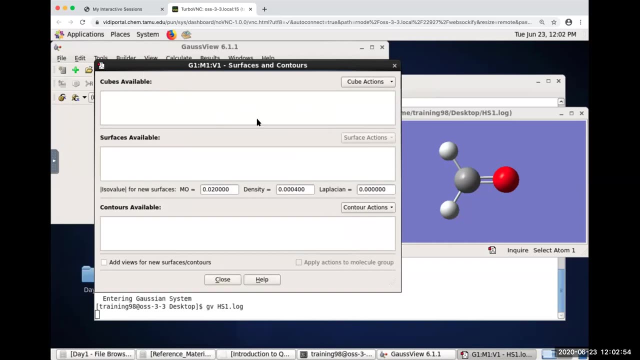 All right. So if you are interested in visualizing some of the other surfaces, you can come in here and look at under the results, surfaces and contours. okay, Yeah, okay, So for this part, it's not going to know that the checkpoint file exists. 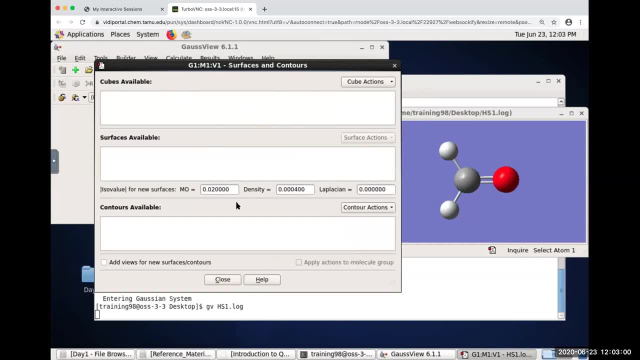 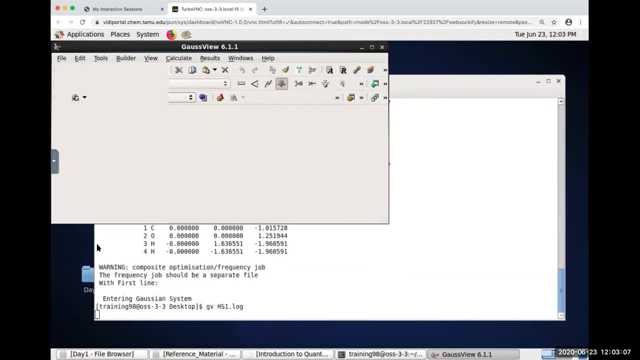 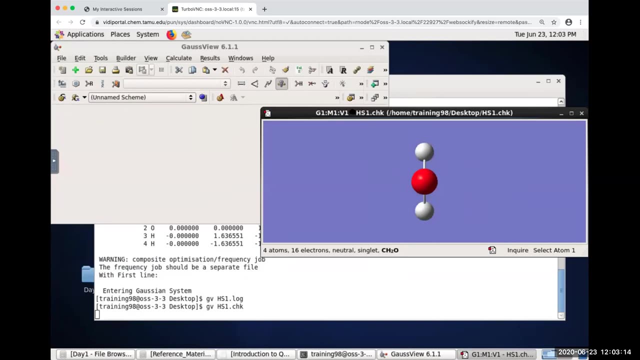 So the only way for you to do the surfaces and contours from this menu is if you load the checkpoint file. okay, So what we're going to do is go ahead and exit and I'm going to load the checkpoint file. Okay, If you do not have a checkpoint file, it's because your calculation either didn't run. 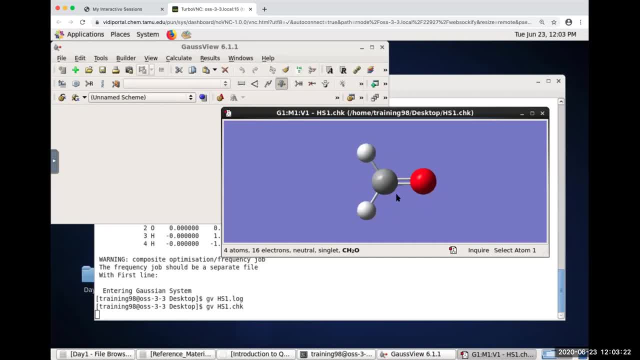 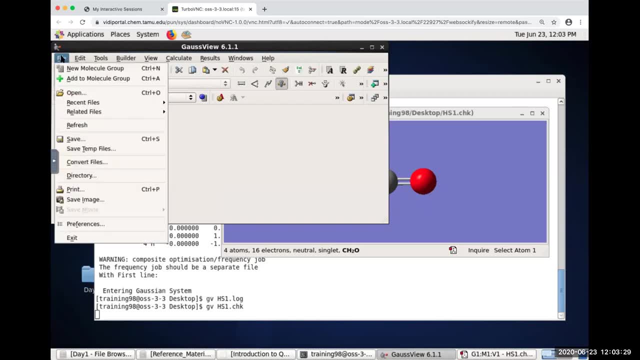 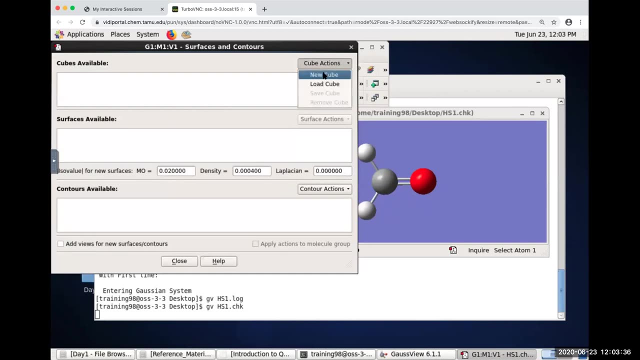 or your percent check line in your input file was not correct and your checkpoint file is not where you think it is, or it got lost, one or the other. okay, So now that I have my checkpoint I can do my results. surfaces, contour, cube, action, new cube. Instead of doing a molecular 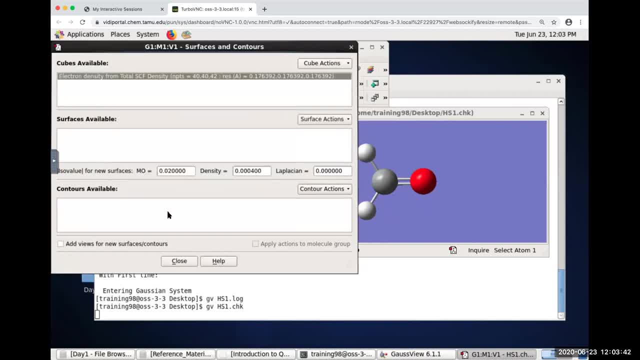 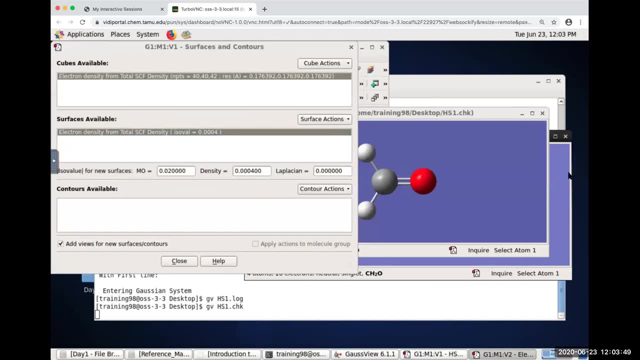 orbital. I'm going to do total density and click, okay, And now I have a cube for that. I generally turn on, add new views, and now I want a new surface, and here is my density: okay, with a surface that has an ISO value of 0.0004.. Okay, Now what I want to do is I want to 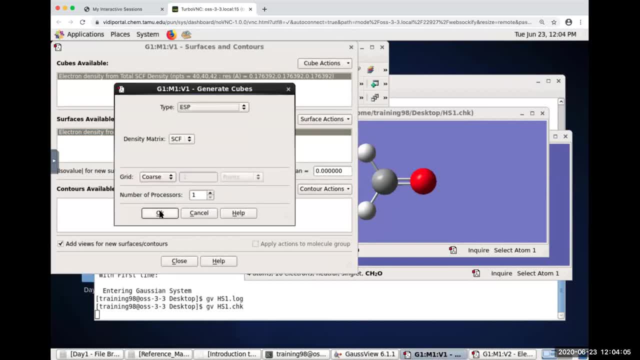 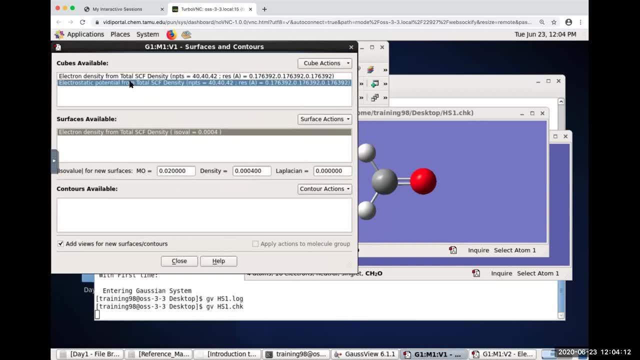 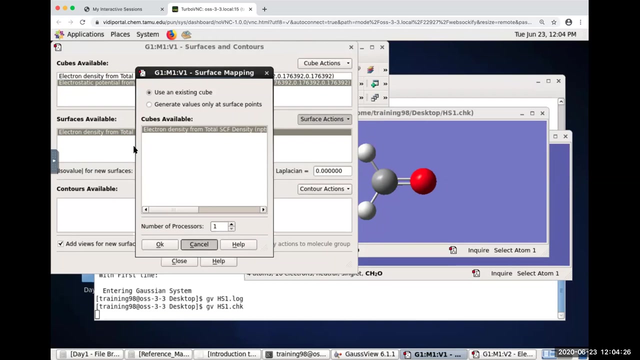 new cube and I want to do electrostatic potential. So now I have electrostatic potential, Okay, And I need to select that one, Okay, And I want this one selected and I want new mapped surface. No, I did that backwards, Sorry. I need the density selected and surface action. 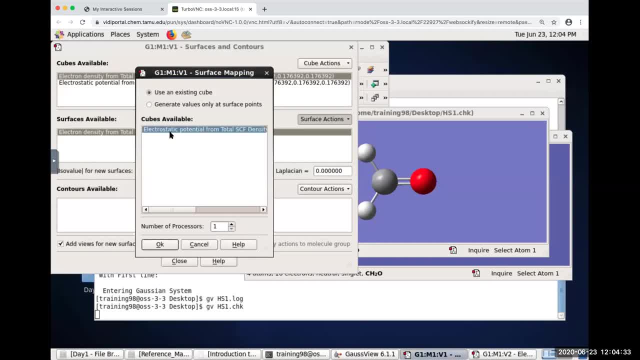 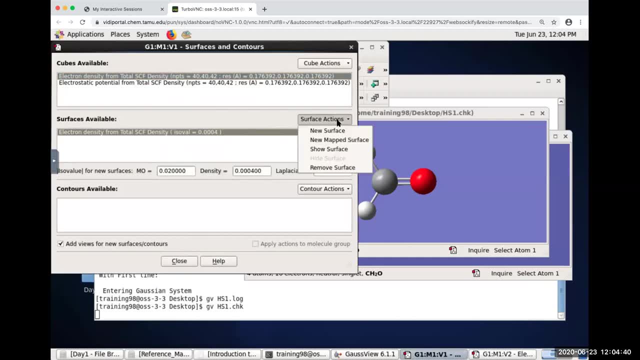 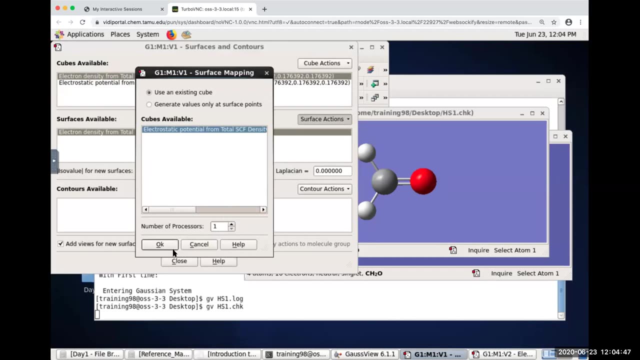 new map surface and I'm mapping the electrostatic potential on the density. Okay, So let me do that one more time: Select the density, surface, action- new map surface, the cube available, You need the electrostatic potential and then you click okay. 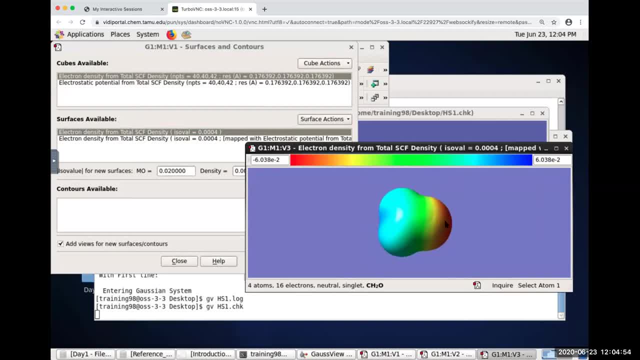 And here is where you get the nice pretty electrostatic potential, where we have an electronegative region, where the red is, and the electropositive region, And we're going to talk more about what this means, But this is the protocol that you go through to visualize these.